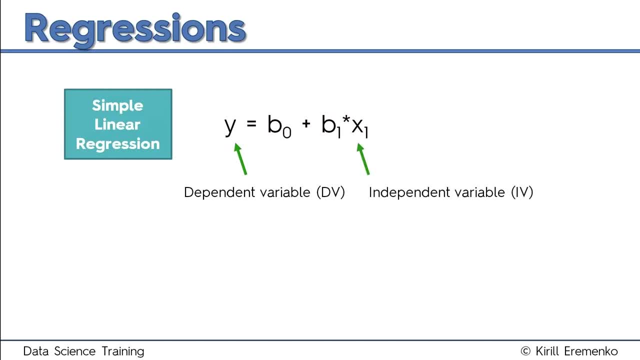 you can understand how it depends on something else. x is your independent variable. In this case, in the Simple Linear Regression, we only have one independent variable, So we don't even have to call it x1.. We could just call it x And this is the variable that is. you're assuming that it is. 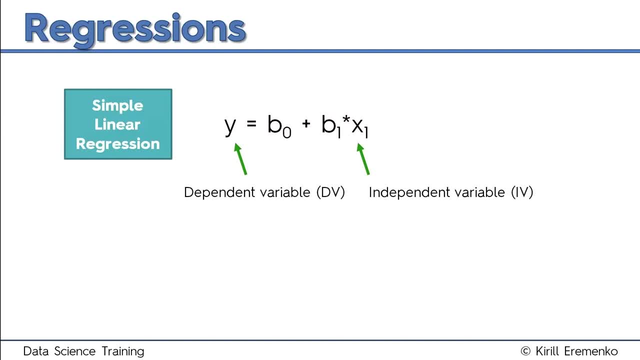 causing the dependent variable to change. Or, as we will learn further, sometimes that independent variable might not be a direct causative factor, but it's still. there might be an implied association between the two And in that case you're trying to figure out this association. Then b1 is the coefficient for the independent. 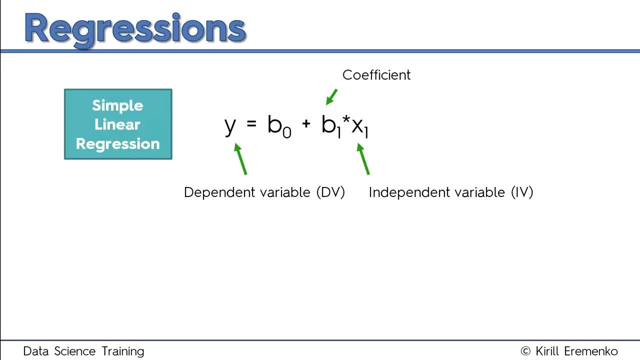 variable And it kind of says how, the effect or how a change in x1,, a unit change in x1,- and we'll be talking about this a lot- unit changes, a unit change in x1, how that affects a unit change in y. So it's kind of think of it as the translator or the multiplier or something. 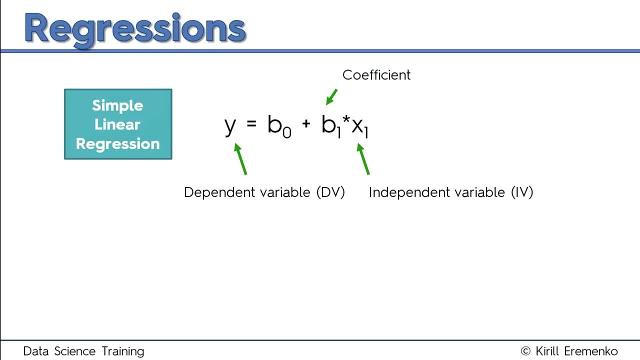 like that. that's the connector between y and x1. So you can't just say, you can't always say, x1 is directly proportional, There is well. you can't just say y. the change in x is always equal to the change. 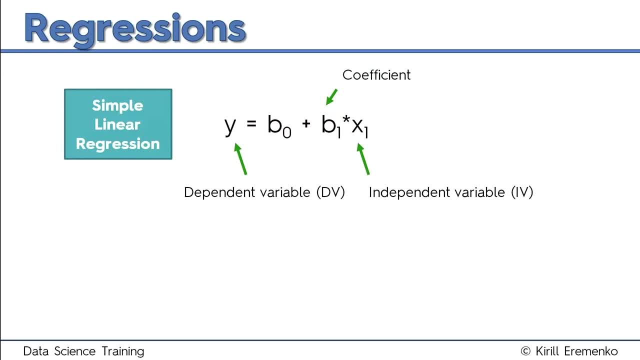 in y There might be this coefficient of proportion, to which proportion that change is inflated or deflated, And b0 is the constant. So it's a constant term, And we'll talk about the constant just in a few seconds. So now let's look at the Simple Linear Regression, because it's the easiest. 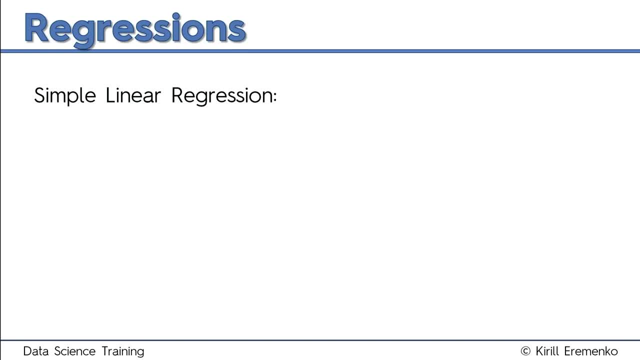 way to do it. So let's look at the Simple Linear Regression because it's the easiest way to do it. So let's look at the Simple Linear Regression because it's the easiest way to do it. So here we've got the y and x axis. Let's look at that specific example where we have experience and 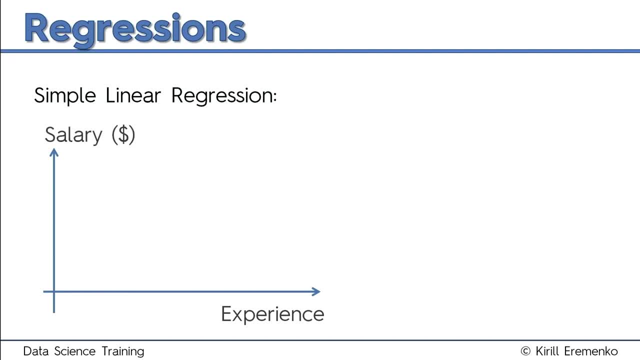 salary. So experience is going to be our horizontal axis, Salary is our vertical axis, And we want to understand how people's salary depends on their experience. Well, what we do in regression is we don't just come up with a theory, We look at the evidence, We look at the 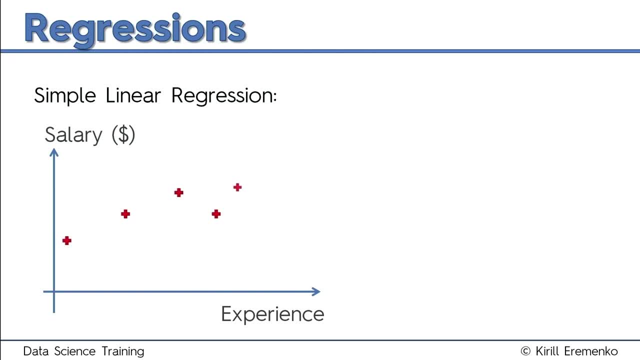 live hard facts. So here are some observations we've had. So in a certain company, this is how salaries are distributed among people who have different levels of experience, And what a regression does is so. that's the formula for regression. In our case it'll change to salary. 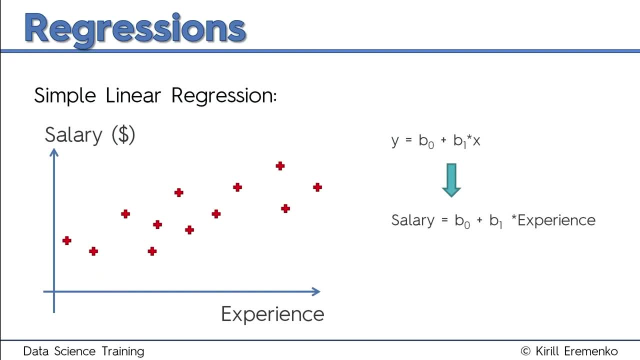 equals b0 plus b1 times experience, And what that essentially means is just putting a line through your chart that best fits this data- And we'll talk about best fitting in the next tutorial, when we're talking about ordinary least squares. But for now, this is the chart. this is the line that 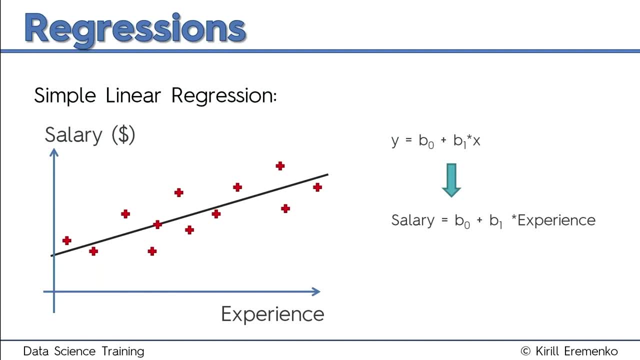 best fits this data and even looks the same. It's quite hard to draw a line that fits this data better, And the assumption here is it's impossible. This is the best line For now. let's focus on the coefficient and the constant. 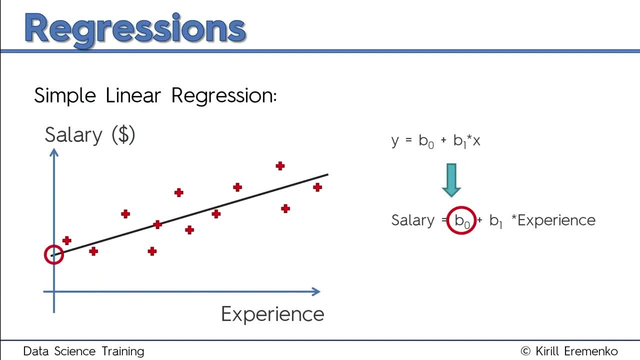 So what does the constant mean here? Well, the constant actually means the point where the line crosses the vertical axis, And let's say it's $30,000.. What does that mean? Well, it means that when experience is zero, so when, as you see, on the horizontal axis, 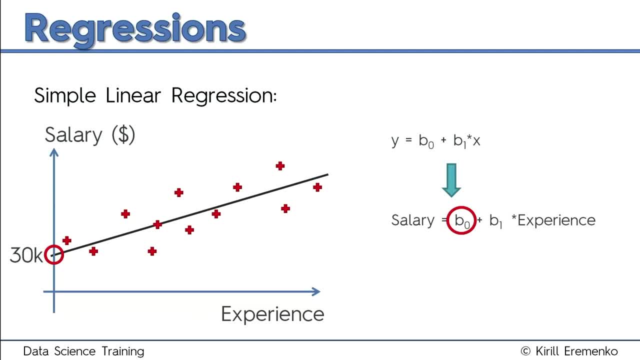 when experience is at zero, then in the formula on the right you can see that the second part b1 times experience becomes zero. So salary equals b0.. That means that salary will equal to $30,000 when a person has no experience. So as soon as somebody is fresh from university and joins this 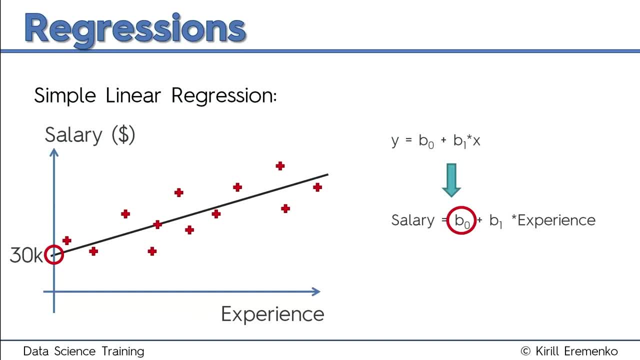 company. most likely they will have a salary about $30,000.. There'll be some confidence intervals there, but we won't go into that right now. Just we can say that according to this model, the first person will be probably getting paid $30,000.. Now what is b1?? B1 is the slope of the 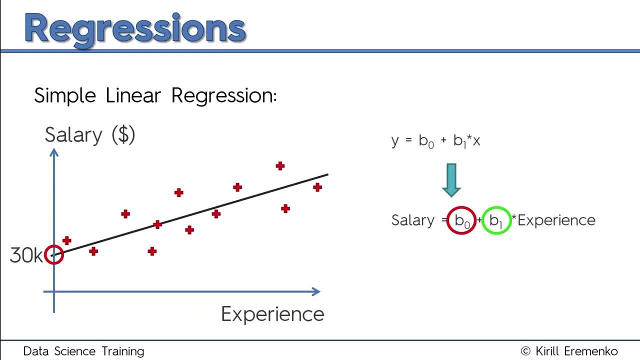 line, And so the steeper the line, the more money you get per extra year of experience. Let's look at this in this particular example. Let's say somebody went from I don't know, maybe four to five years experience, Right, So then to understand how his salary will. increase. you have to project this onto the line and then project that onto the salary, which is the number of hours that he spent on the line, And then, if he is a senior, he is probably going to get more money than he is a senior, And so the ratio of the two is going to be the number of hours that 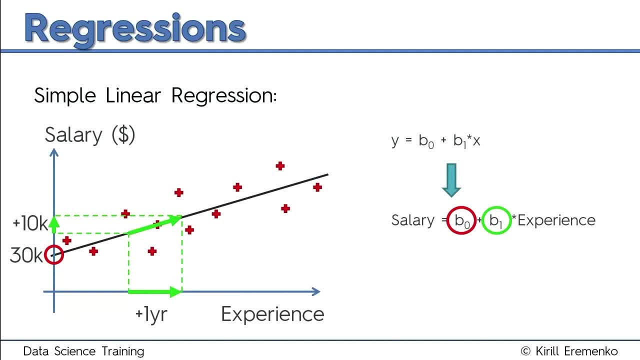 he's spent on the line And the ratio of the two is going to be the number of hours that he has spent on the line. that onto the salary access, and you can see that here for one year experience the person will get an extra ten thousand dollars on top of his salary. so 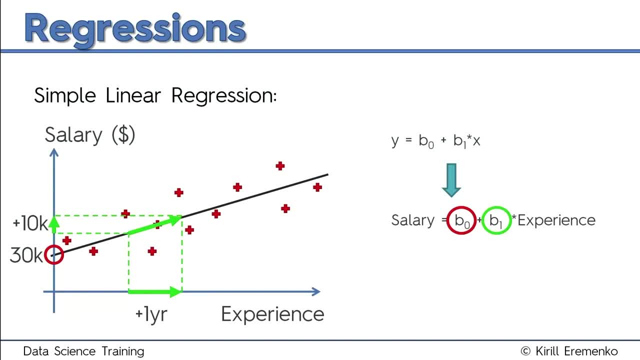 if the coefficient p1 is less than, the slope will be less and that means the salary increase will be less per every year of experience. if the slope is greater, then that means the experience will yield a more increase in salary, and that's pretty much it. that's how a simple linear regression works. so the 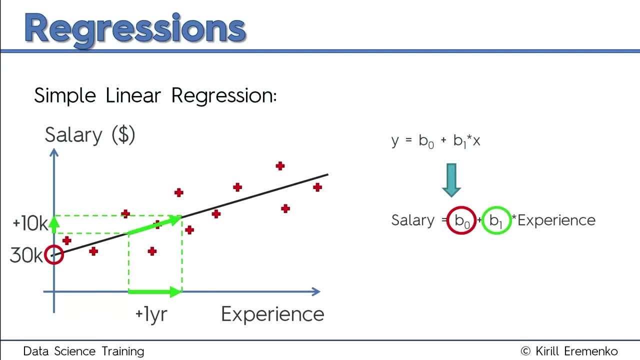 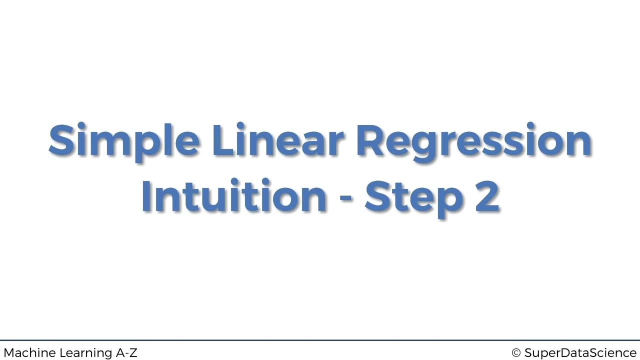 core goal here is that we're not just drawing a line theoretically that we came up with somehow. we're actually using observations that we have to find the best fitting line, and what a best fitting line is. today we'll find out how to find that best fitting line, or in fact how the simple linear regression. 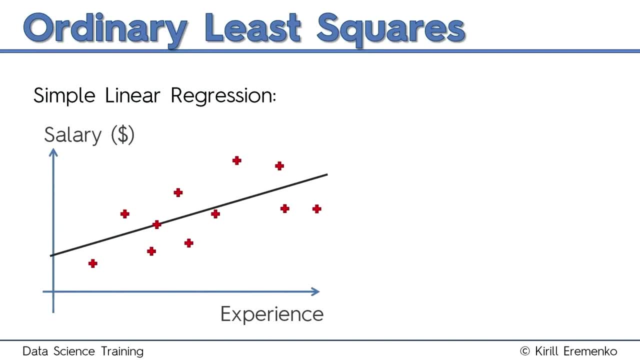 finds that line for you. so here's our simple linear regression: the same chart, salary versus experience, salary versus experience. we've got these red dots, which represents the actual observations that we have in our data, and we've got the trend line, which represents the best fitting line, or the simple linear regression model. so now let's draw some. 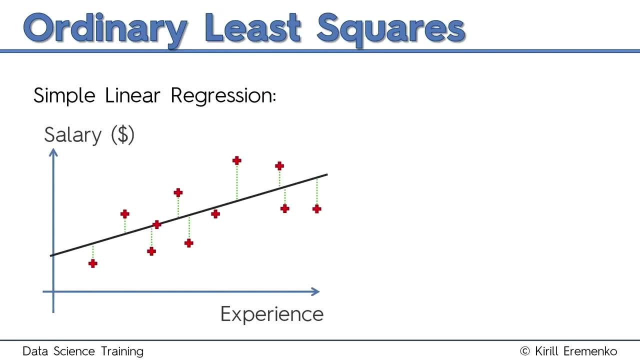 vertical lines from the actual observations to the model, and let's look at one of these specific examples to understand what we're talking about here. so here you can see that the red cross is where that person is sitting at in terms of salary. So let's say, this person with 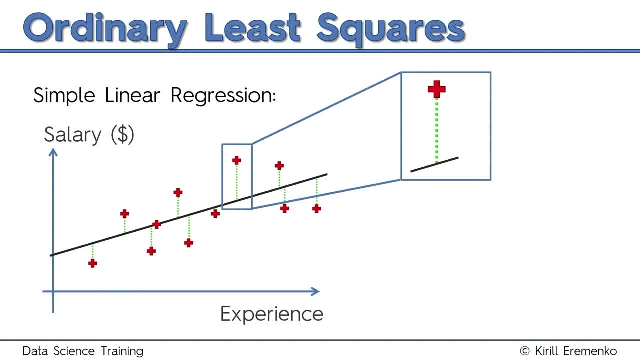 10 years of experience, is earning $100,000.. Well, the model line, so the black line at the bottom. it actually tells us where that person should be sitting according to the model in terms of salary, And according to the model, it should be a bit lower. It should be. 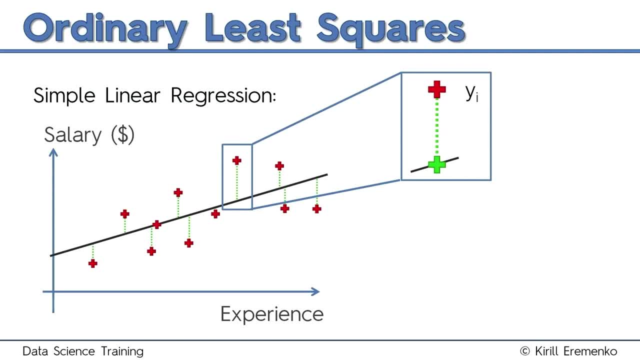 somewhere where that green cross is, which is about maybe, let's say, $80,000.. So now the red cross is called YI, so Y of the subscript I and that is the actual observation. The green cross is called YI hat and that is the modeled observation or the modeled value. So 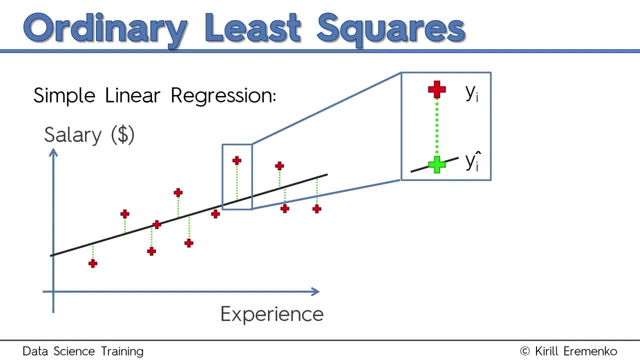 basically, with that level of experience, where does the model predict that he would be earning? And so the green line, therefore, is the difference between what he's actually earning and what he should be earning or not should be what he's modeled to be earning. 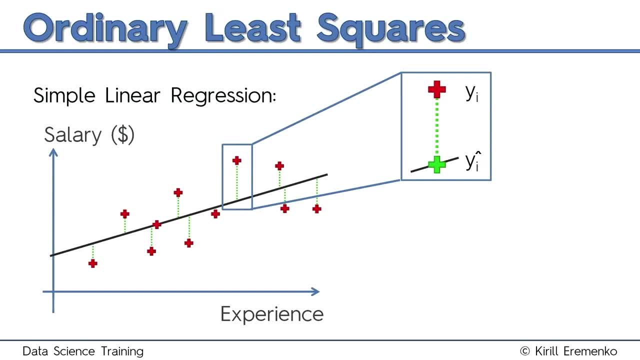 So, therefore, the green line, it will be the same regardless of what dependent variable you have, whether it's salary, whether it's grade at school, whatever. So it's the difference between the observed and the modeled for that level of independent variable. 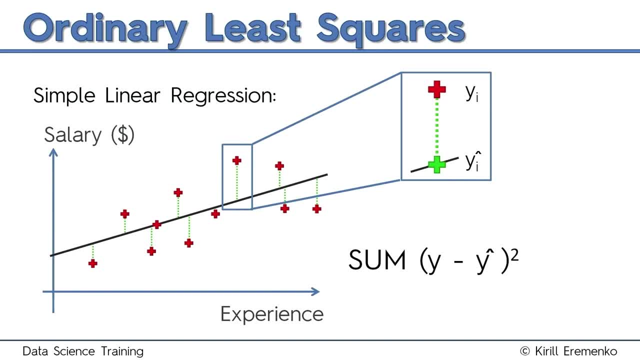 Now, to get this best fitting line, what is done is you take the sum. you take each one of those green lines or those distances, you square them and then you take the sum of those squares. Once you have the sum of the squares, you take the sum of the squares and then you take the sum of. 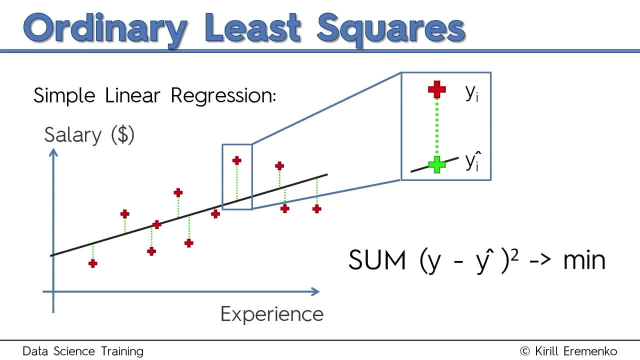 the squares, you gotta find the minimum. So, basically, what a simple linear regression does is it draws lots and lots and lots of these lines, these trend lines. Well, this is like a simplistic way of imagining it. The linear regression draws all these, all possible trend lines through your 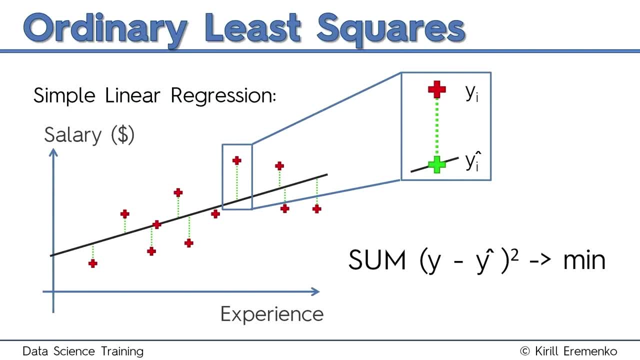 data and counts the sum of those squares every single time and it records it somewhere in a file or something like that. Then it finds the minimum one, So it looks for the minimum sum of squares. It finds a line which has the smallest sum of squares possible And that line will be the best fitting line, And that is. 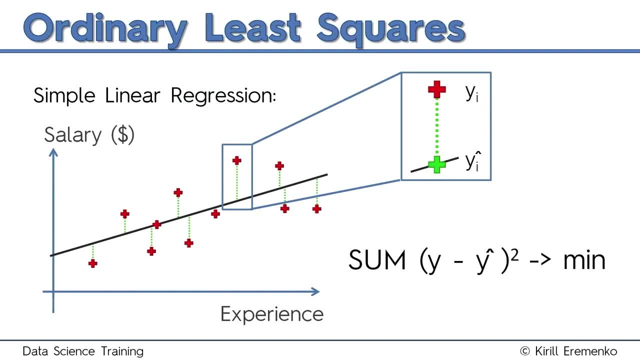 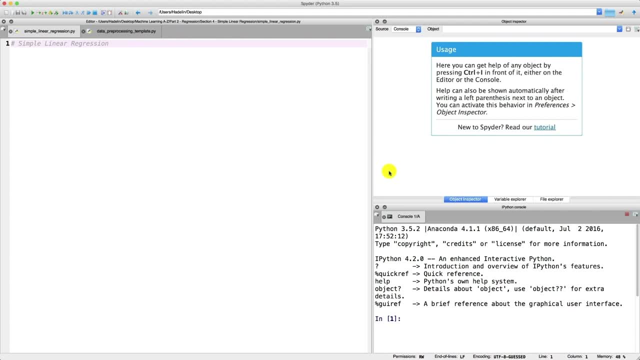 called the ordinary least squares method. So that's how the simple linear regression works. Hello and welcome to this Python tutorial. I'm super excited because we are going to implement the very first model of machine learning. We're going to start with the most simple one. It's the 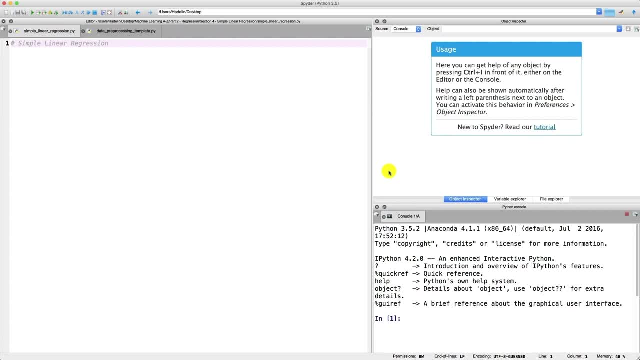 simple linear regression model, And it's going to be the most simple one. So let's get started. So let's do it right now and let's do it on Python. So the first step of making a model is to preprocess the data. 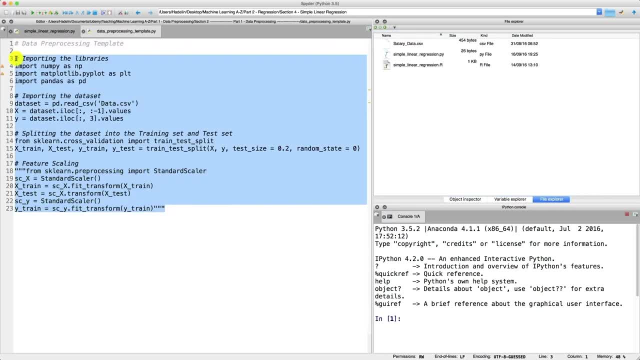 So let's just copy all this. That's the data preprocessing template. Let's copy this and let's put it in our simple linear regression Python file And let's paste it here And now. we need to change a few things. Well, first we need to change the name of our dataset. 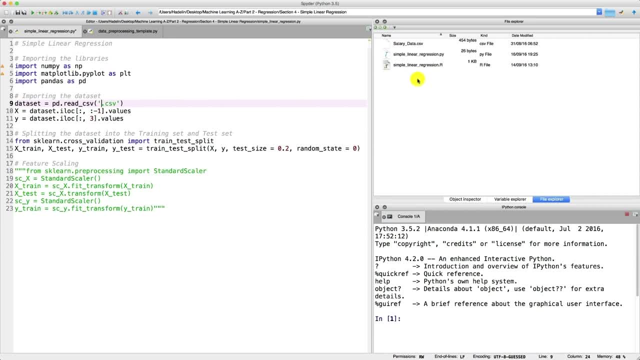 Here it's not datacsv but salariedatacsv, So let's change it right now: salariedatacsv. And now let's see what we need to change. Okay, so first let's import the libraries to get the essential tools we will need to build our model. 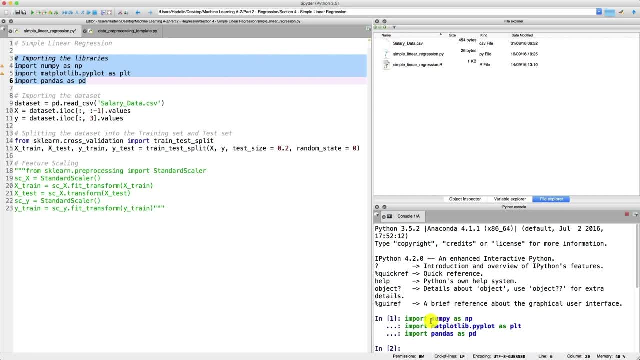 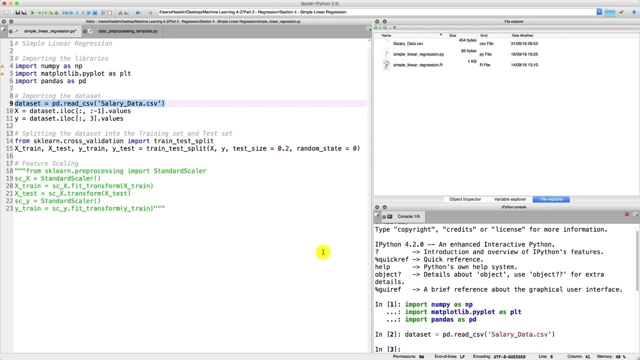 And here, as you can see in the IPython console, the libraries are well imported. And now let's select this line and execute to have a look at our dataset. So, as you can see here, the dataset is well imported. And now to have a look at it. 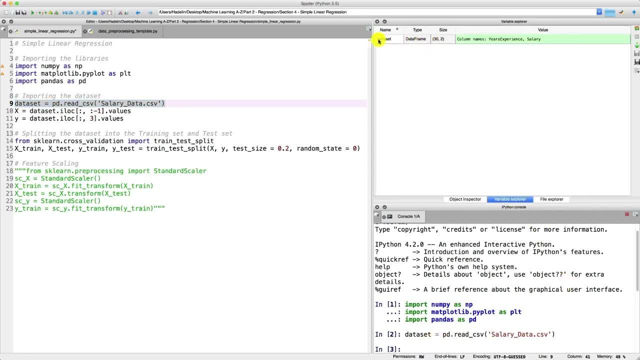 we need to go to our database. We go to Variable Explorer And then appears here the dataset. So let's double click on it And let's explain the problem. So first of all let's perhaps change the format, because we have the scientific notation. 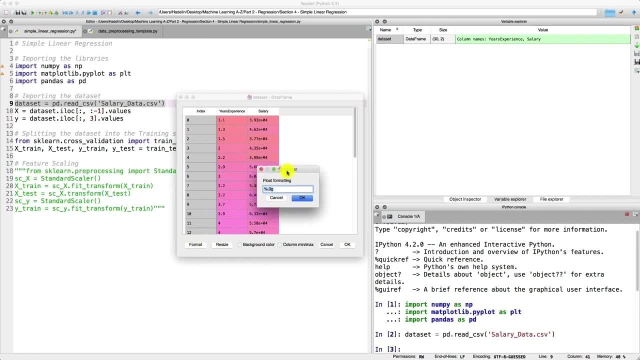 Maybe we would prefer something like with no decimal and regular floats with no decimal. So to do this, we need to change this 3 here, which is the number of decimals, by 0, and this g by f, And then you'll see that if I click OK. 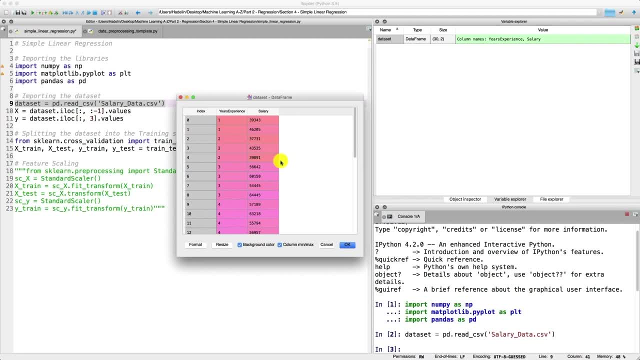 I'll get my salaries in this format, Which is, I think, better. So OK, so this dataset contains two columns: the years experience and the salary. So basically, these are information of employees in a company. The first column, years experience, gives the number of years of experience each employee has in the company. 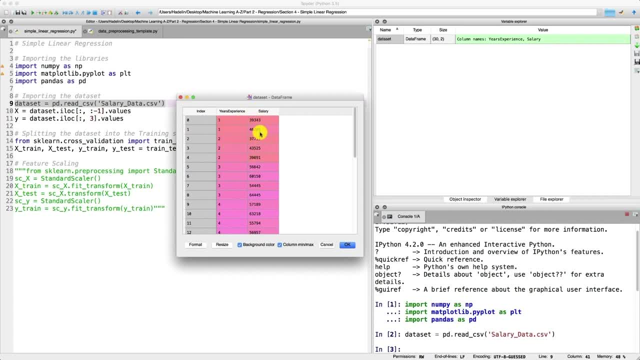 and its respective salary in the salary column, And so we have 30 observations, that is, 30 employees for which we have those informations, Because, as you can see, the index starts at 0 here, And so what we'll do here is that we will train a simple linear regression model. 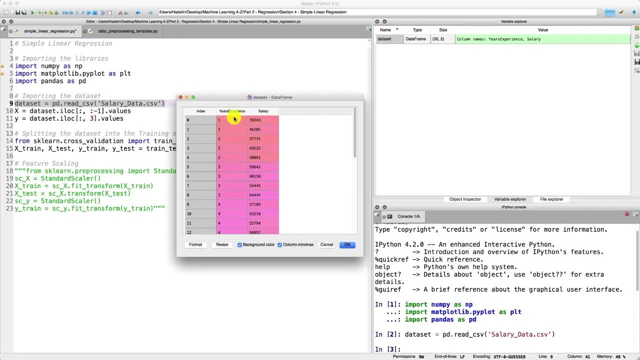 that will learn the correlations between the number of years of experience each employee has in the company and its salary. And by understanding those correlations between the number of years of experience and the salary, then the model will be able to give some predictions for each of the numbers of years of experience here. 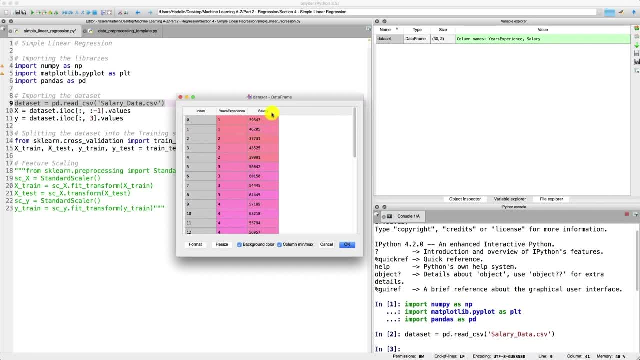 And you're going to see how the predictions will be closed to the true results, which are the true salaries. So we will compare the true salaries with the predicted salaries. OK, and now let's see what we need to change here for x and y. 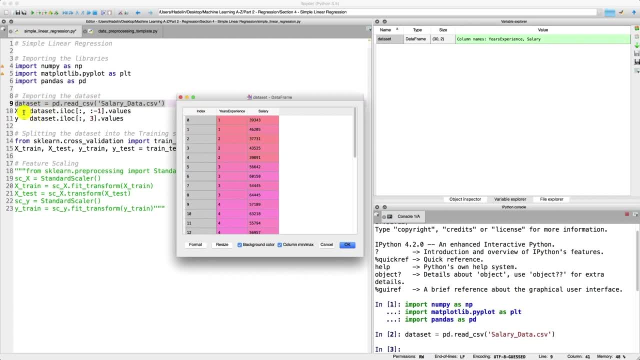 So, as a reminder, x is the matrix of features, that is the matrix of independent variable. Here the independent variable is this variable, here the years, experience, the number of years of experience, And then the dependent variable is the salary. 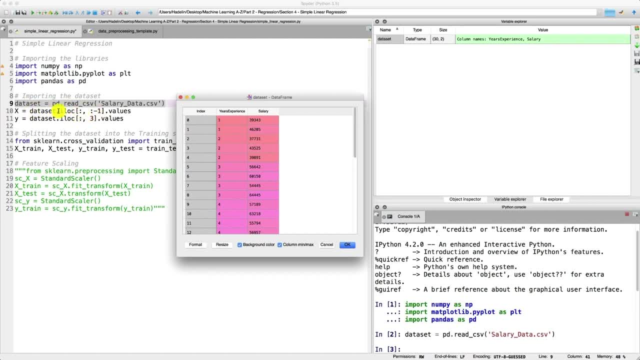 So our matrix of features here, which is, you know, taking the dataset and removing the last column of the dataset, that is, the salary column, with this minus one here, will contain only one column, which will be the number of years of experience. 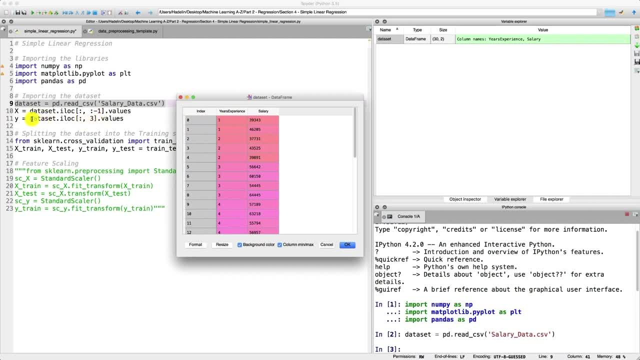 But then we need to change the index here for y because remember, in our data example in the data preprocessing part the dependent variable was on the fourth column. So since indexes in Python start at zero, then it had index three, But here you can see that the dependent variable is the second column. 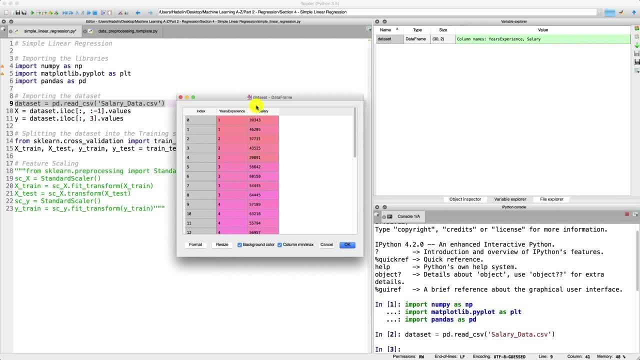 And so since indexes in Python start at zero, that means that this column here has index one. So here, since we need to put the index of the dependent variable column, then that means we need to put one, And then we're all good. 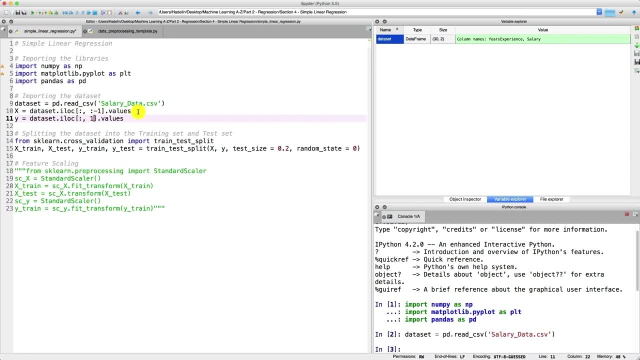 We're ready to create our matrix of features, which is here a matrix of only one column, and our dependent variable vector. So let's do this. You'll see I'll select this line and press Command and Control plus Enter to execute. Here it is. 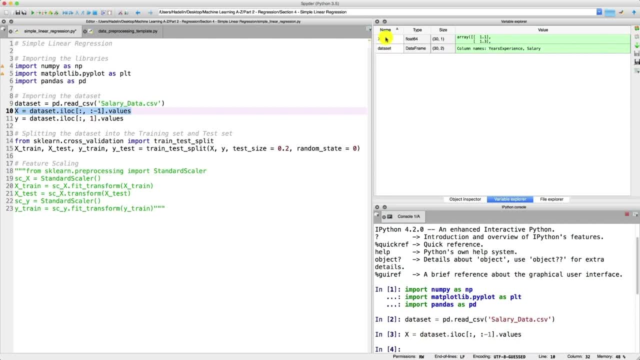 The matrix of features x is created. Let's have a look. So, as I just told you, this matrix contains only one column. You can see here, actually, that it contains 30 lines and one column. So that's our matrix of independent variable. 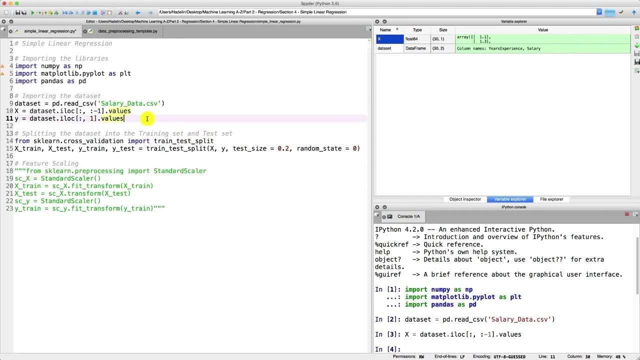 And now let's create our dependent variable vector. And now that we corrected the index here, it should be all fine. So let's select this and press Command and Control plus Enter to execute. Here it is. Let's have a look at y. 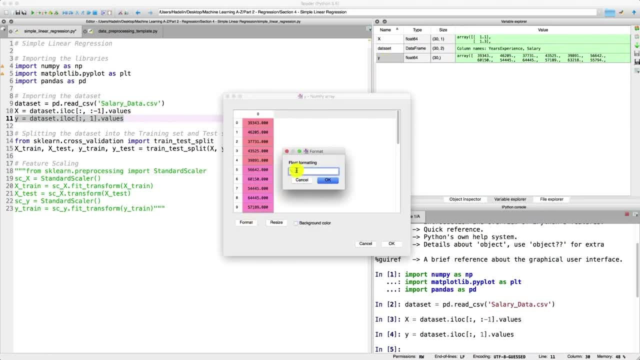 And here is y. We can change the format again and replace this 3 by 0 to have the salaries in this format. That's better And that's all our salaries. and this column is the dependent variable vector And, as you can see, 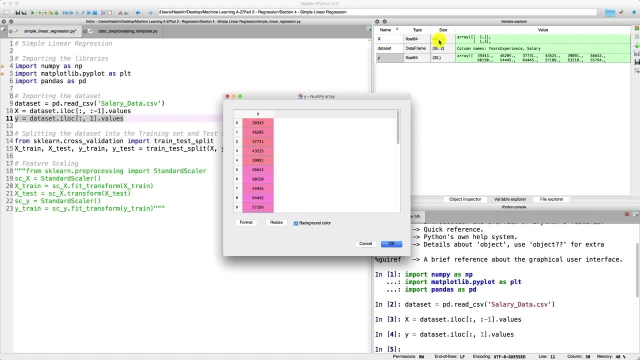 we can clearly make the difference here between the matrix of features and the vector here, because, as you can see, there is this 1 here that tells that this is a matrix that has one column, And here we don't have anything after the comma. that means that it's a vector. 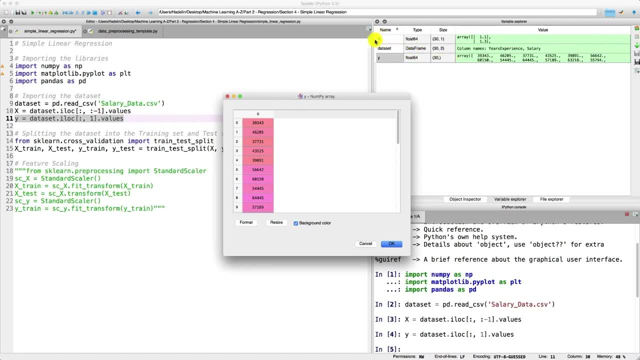 So you have to make the distinction between the fact that this x here is a matrix, because it's the matrix of features, the matrix of independent variable, and y here is a vector, since it's the vector of the dependent variable. So let's click OK. 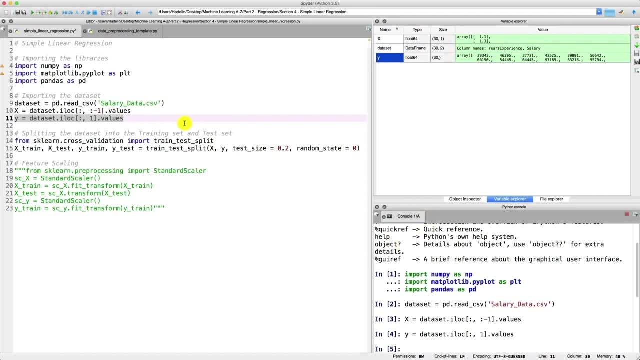 and now we're all good. So now we're ready to move on to the next sub-step of the data pre-processing first step of our model, And this is to split the data set into the training set and the test set. So let's see, we have 30 observations. 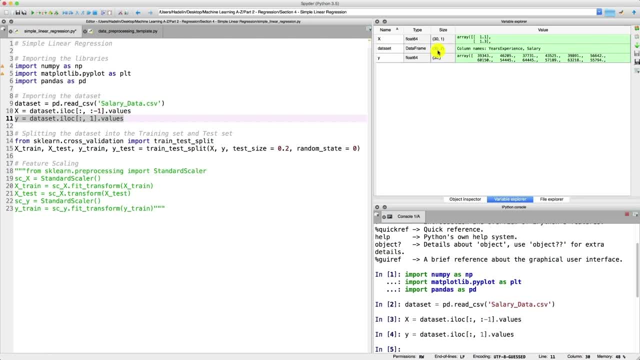 So a good split would be to have, for example, 20 observations in a training set and 10 observations in a test set. Let's pick that split, even if we recommend in general more like an 80-20% split. But here we're making a simple model. 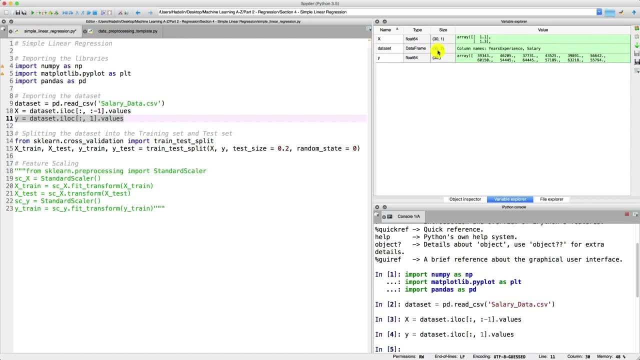 so we can select 20 observations to go to the training set and 10 to go to the test set. So that means that for the test size here we need to input 1 third. So that way 1 third of 30 equals 10 observations. 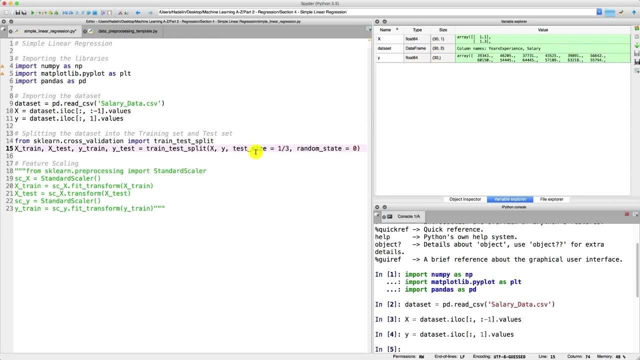 will go to the test set And that's it. That's all we need to do Now. we're ready to change. Now we're ready to make the split of the data set into the training set and the test set, And remember this random state parameter here. 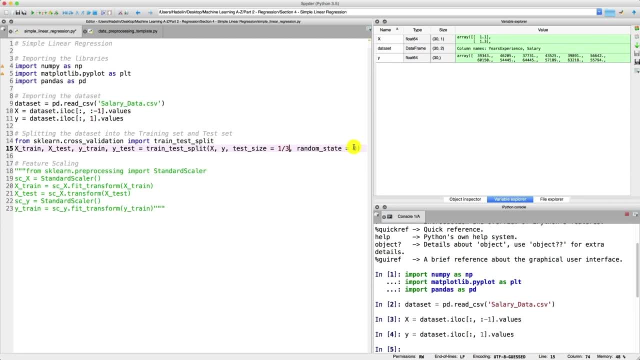 set to 0 is here so that we all get the same results, because there are some random factors in the algorithm, So it's better for the learning experience if we all have the same results. So let's select this. It's all ready now. 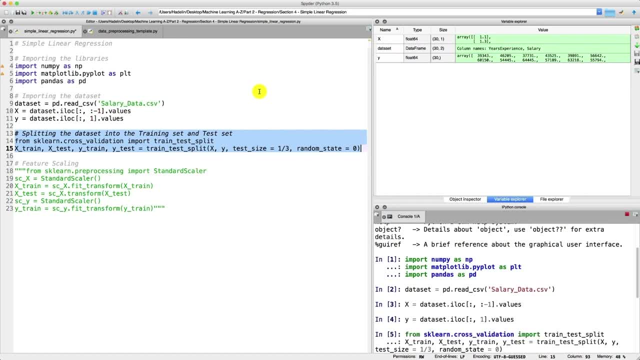 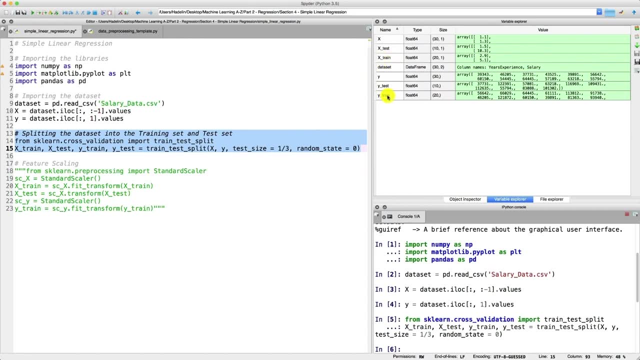 Let's select this section and press Command and Control plus Enter to execute. And, as you can see, now our training set, composed of X train and Y train, is created, And our test set, composed of X test and Y test, is created as well. So let's have a look at them. 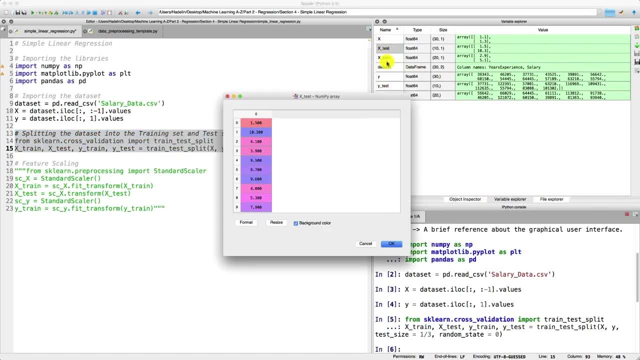 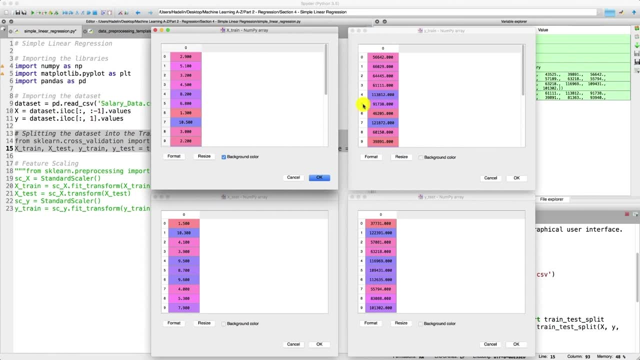 X train, Y train, X test and Y test. Okay, so these two sets above are composing the training set, because it contains X train, the matrix of independent variable, and Y train, the dependent variable vector for the training set. And below is the test set, composed of X test. 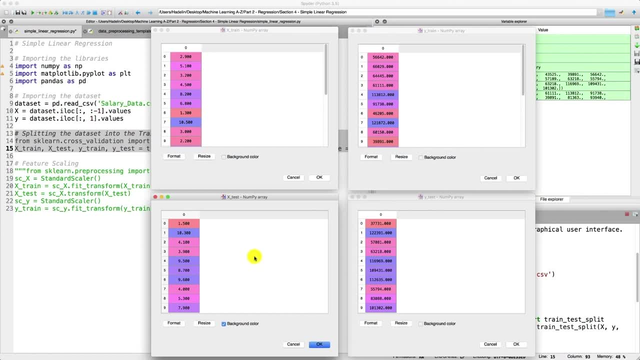 the matrix of independent variable for the test set and Y test the dependent variable vector. And so what happens is that we are going to train our model on the training set here. That means that our model will learn the correlations between X train here- and Y train. 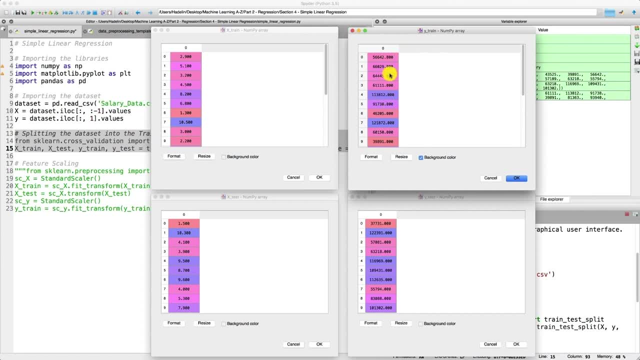 so that it can later predict the results of the dependent variable, the salaries, based on these informations. here And then, once our model is trained on the training set by having learned all the correlations between these two variables, we will test its performance, its power of prediction. 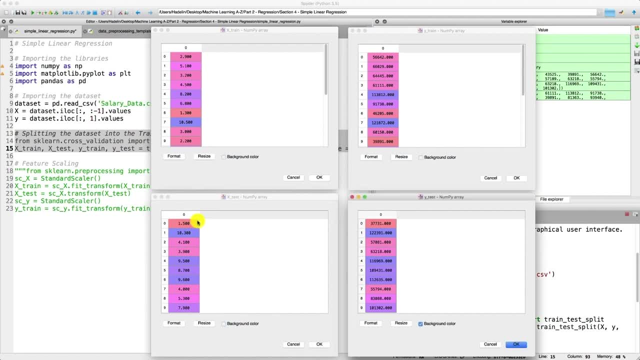 on the test set here. So that means that for each of the test set observations here we will predict the corresponding salary and then we will compare the predicted salary to the real salary, which are the salaries here. So you're going to see that in the next step. 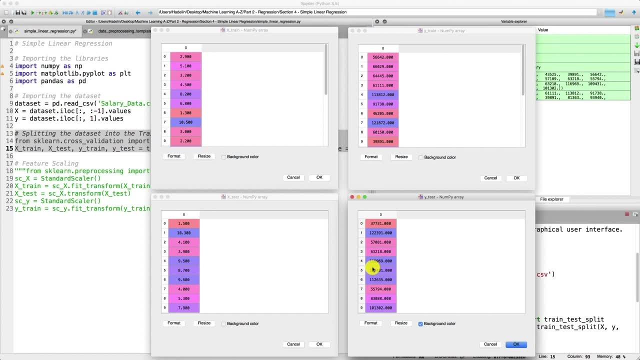 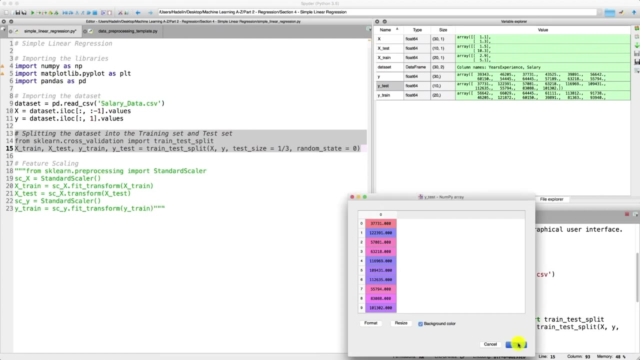 but that's the idea behind making a model, making any machine learning model, We're training the model on the training set. that means that our model learns on the training set and then we're testing its performance on the test set. Okay, so let's click OK to close the windows here. 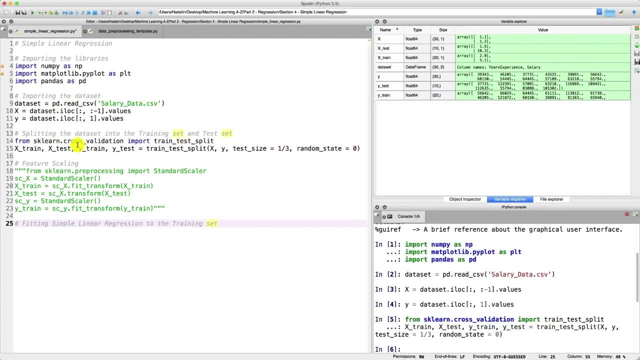 and now let's move on to the next step. That's what we did in the first step. Now the data is all well pre-processed. We have our training set here, with X train and Y train, and our test set, composed of X test and Y test. 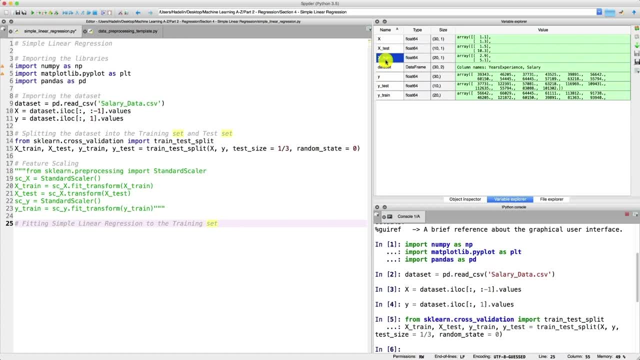 and we didn't have to apply feature scaling. as you can see on X train. here We have the numbers of years of experience as they were originally, and that's because the library that we're going to choose to build our simple linear regression model, will take care of that for us. 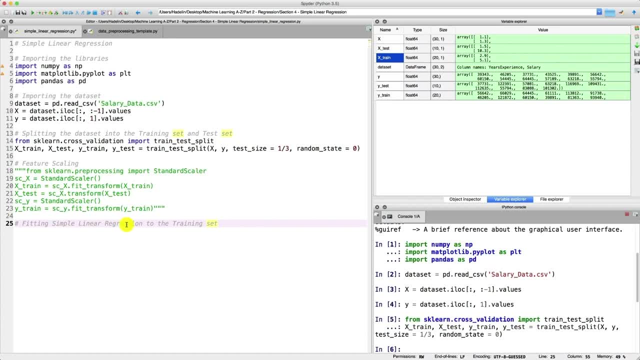 And, speaking of library, that's what we're going to do in this tutorial, because we are going to fit the simple linear regression model to the training set and to do this, we're going to use this specific library that will do the job for us, and you will see how easy it is. 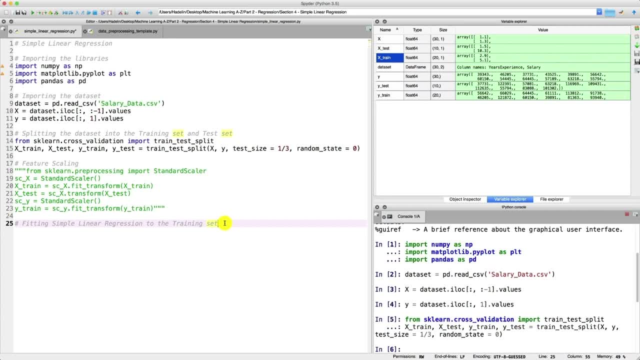 to fit the simple linear regression model to the training set. So let's do this right now. The first thing that we need to do is obviously to import this specific library, and so we're going to import it from scikit-learn, which contains a great deal of libraries and tools. 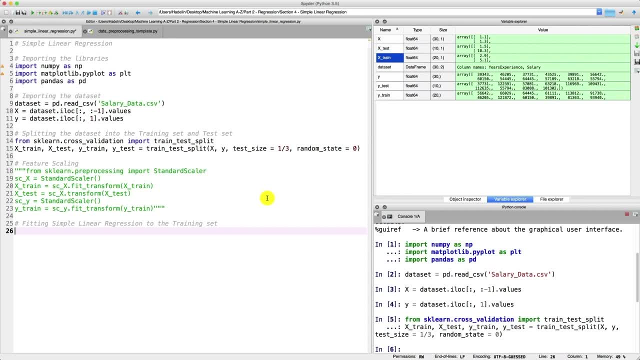 to make machine learning models, and so the library that we're going to use for simple linear regression is the linear model library from scikit-learn, And then in this library we are going to import a class which is the linear regression class, and then what will happen is the following thing: 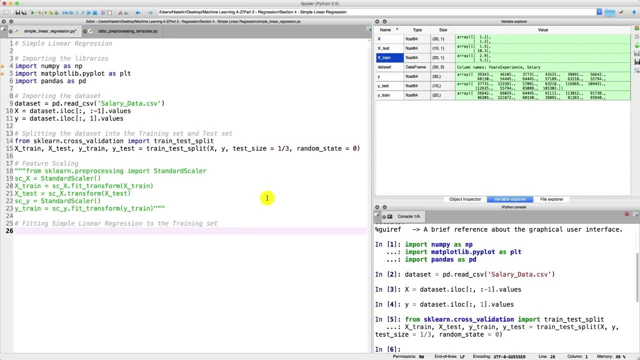 we are going to create an object of the linear regression class, and this object will actually be the regressor, the simple linear regressor, and so we're going to call this object regressor, simply because it's going to be the regressor that we will fit to the training set. 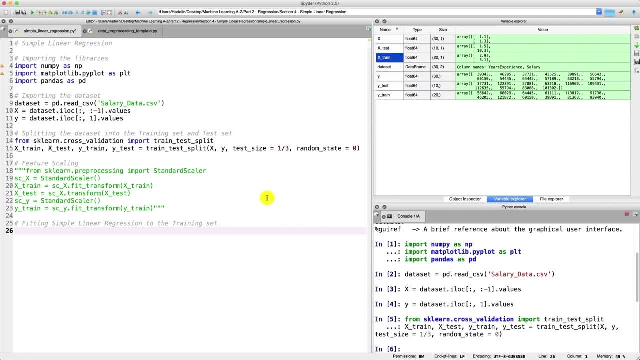 and actually, in order to fit it to the training set, we will use something called a method, because the linear regression class contains several methods and one of them is the fit method. and this method is like a tool, a function that will fit your regressor object. 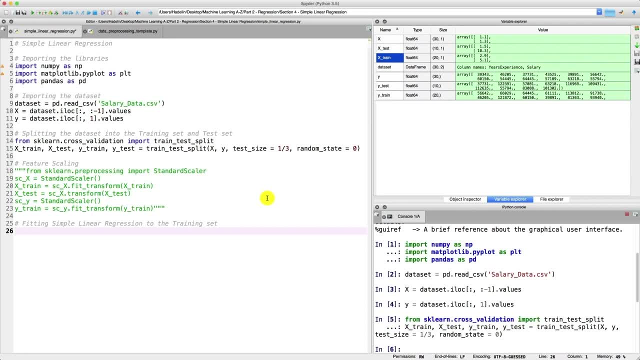 that we will create to the training set. so let's write the code and everything will be all clear. so the first thing that we need to do is to import the linear regression class. so let's do this. so, since we are importing this class from scikit-learn linear model library, 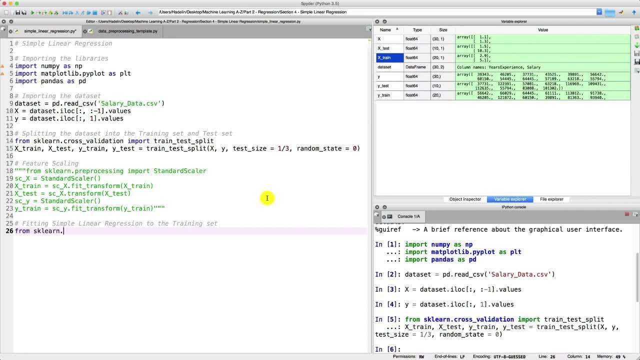 we will first write from sklearn that linear underscore model which is the name of the library, and so from this library we are going to import the linear regression class, and the linear regression class is spelled this way: with capital L in linear and capital R in regression: no space. 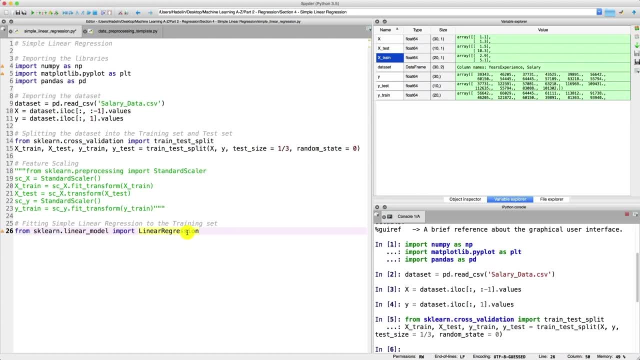 here it is. that's your class, the linear regression class, and so now we are going to create an object of this linear regression class that we will call regressor. so here I am writing regressor, and that's where I am creating my object of the linear regression class. 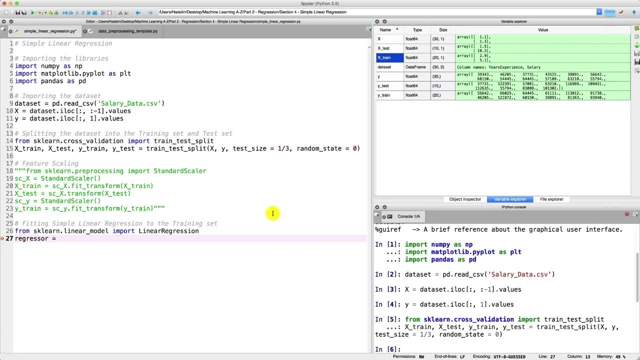 and to create an object of the class here we need to call the linear regression class and to call it we simply write its name, linear regression, and then we write parenthesis, because by doing this, this is like a function that will return an object of itself, which is actually the regressor. 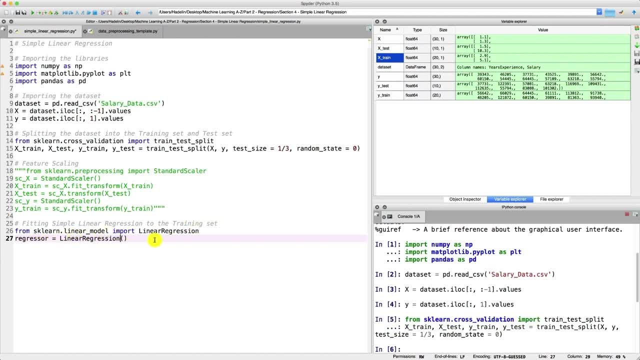 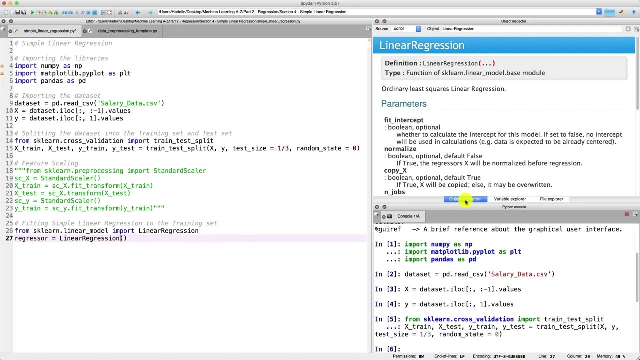 and actually, if we click here at the end of linear regression and if we press command plus I, that will inspect this class and we will be able to get some info about this class. so let's do this, let's press command plus I and here, as you can see in the object, inspector. 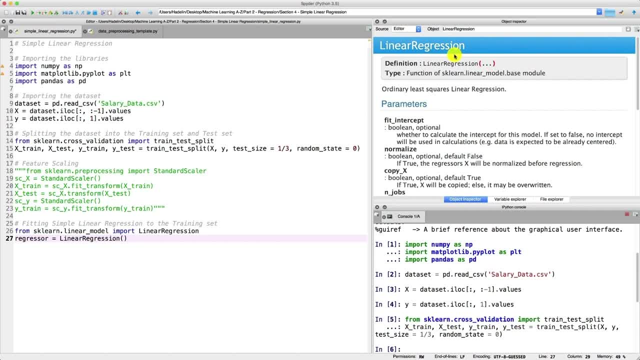 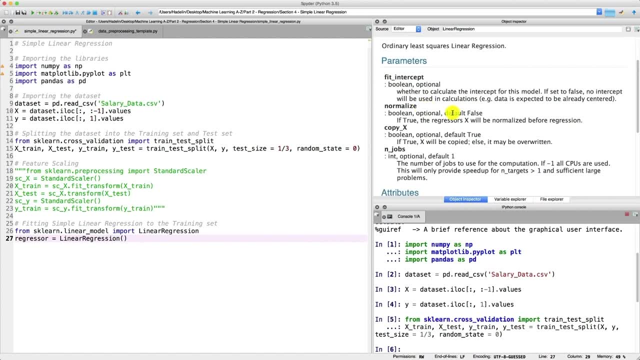 I have some information about the linear regression class, so the main information that we are mostly interested in are the parameters. but here that's just to show you that we can get some information about the class and that there are some parameters to input, but these are not compulsory parameters to input. 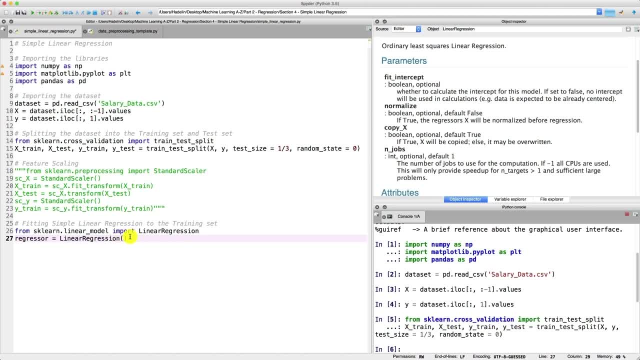 and therefore we will not input any parameters here. we are satisfied with this. with this, we can create a simple linear regression model. we don't need to input the parameters, so that's it. with this simple line, the regressor object is made, and now what we need to do is to fit it. 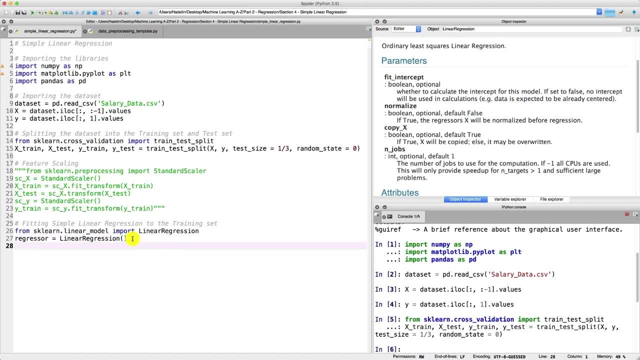 to the training set, and so, as I told you, a class contains some methods, and one of these methods is the fit method, and that's the method we will use to fit the regressor object to our training set. and so, to use this method, we need to first take the object. 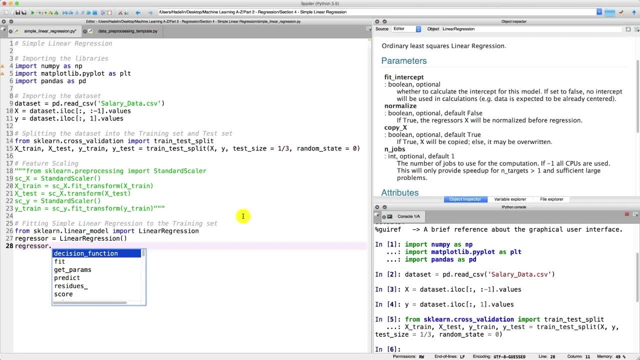 regressor, then, by adding a dot here, we can, as you can see, call the different methods of the linear regression class. these are all the methods, and so the method we want to choose is the fit method, because it's the method that will fit our regressor. object to the training set. 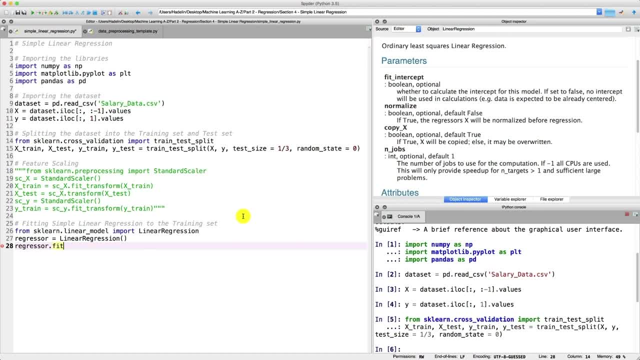 so let's press enter here and now we are taking the fit method, and so now we need to add some parentheses, because we need to specify which dataset we want to fit the regressor to, and of course it's the training set, and remember the training set in Python. 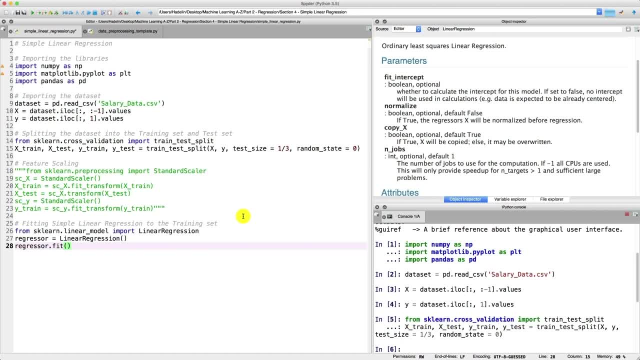 is composed of x train and y train, so here we will need to specify both, and actually we can do the same here. for fit, we can inspect it by pressing command plus i, and, as you can see, this gives the information about the fit method and especially the parameters to input. 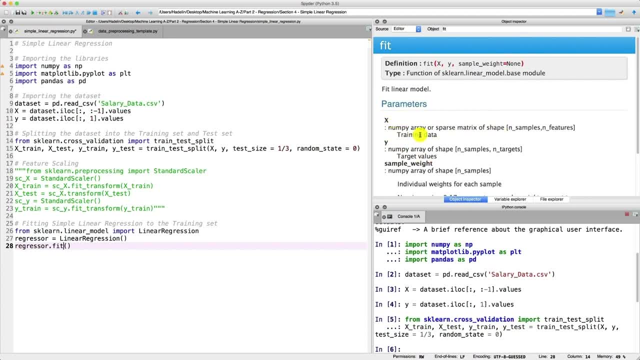 and here you can see that the first parameter is x, which is the training data. and by training data here they mean that it's the matrix of features of the training set, and the matrix of features of the training set is the matrix of the independent variable, that is, x, train. 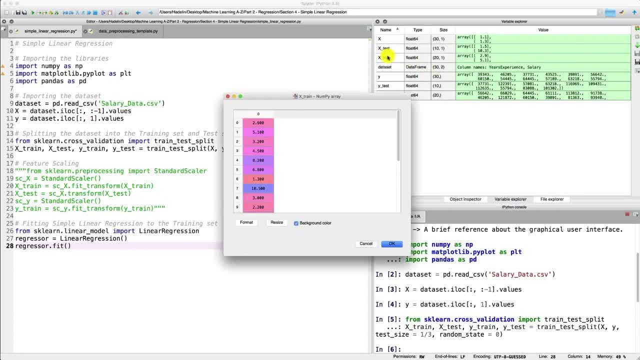 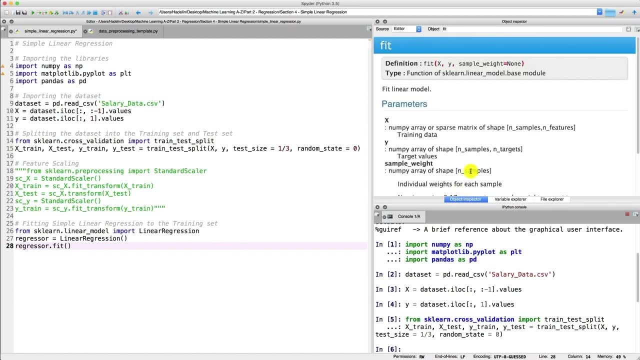 because if we go to variable explorer here, you can see that x train contains the independent variable and only the independent variable, and that's where we want to input for this x here. so that means that the first argument is x train. and then what is the second argument? 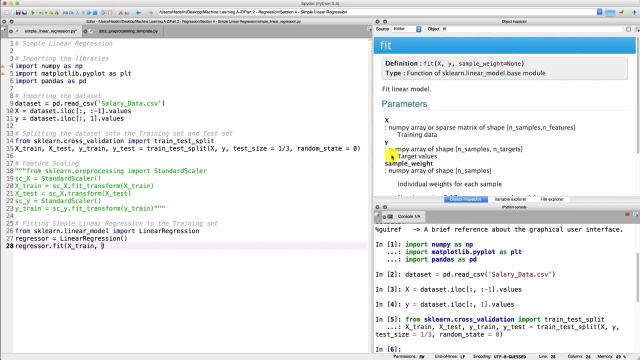 it says that the second argument is y and that y is the target values. so the target values is just another name for dependent variable, because these are the target values that we want to predict and of course this has to be associated to x train here because we are fitting our regressor. 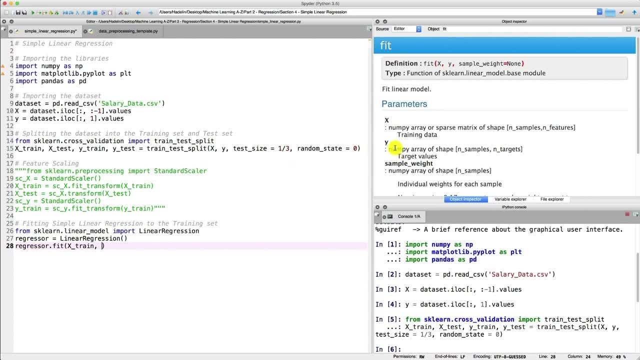 to the training set. so y here is going to be the dependent variable vector of the training set, that is, and y train. so here for the second parameter. we need to input y underscore train, and that's it. this line of code fits your regressor object, which is an object of the linear regression class. 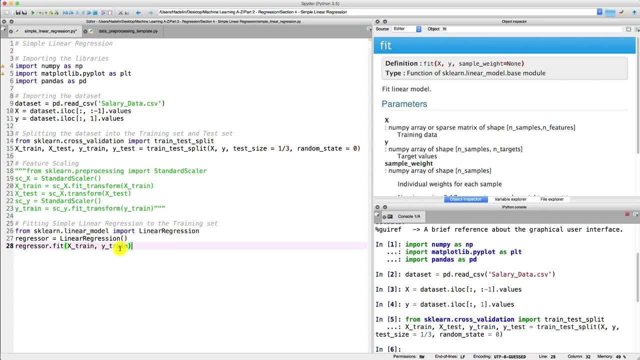 to the training set, composed of x train and y train. and so now this code section is ready, so we are ready to select this and execute, and this will not only create our simple linear regressor, but also it will fit this regressor to our training data. 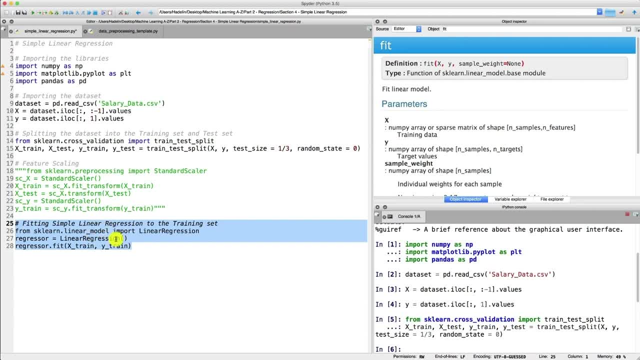 that means that by executing this code section here, our model will already learn the correlations of our training set to learn how it can predict the dependent variable, which is the salary, based on the information of the independent variable, that is, the number of years of experience. so now let's press command or control plus enter. 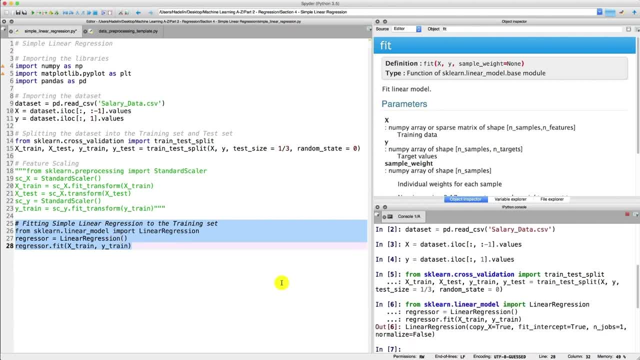 to execute this code section here. and here we go: our simple linear regressor is created and fitted to the training set. so if you want to compare it to machine learning, well, here the machine is the simple linear regression model and learning is the fact that this simple linear regression machine. 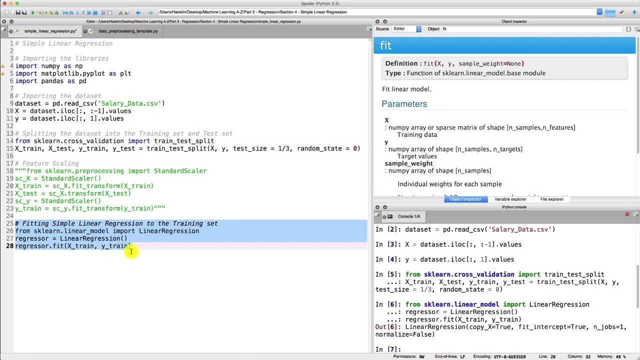 learns on the training set, here composed of x train and y train. so that's what machine learning is. we created a machine which is the regressor here, the simple linear regressor, and we made this machine learn on the training set to understand the correlations between the experience and the salary. 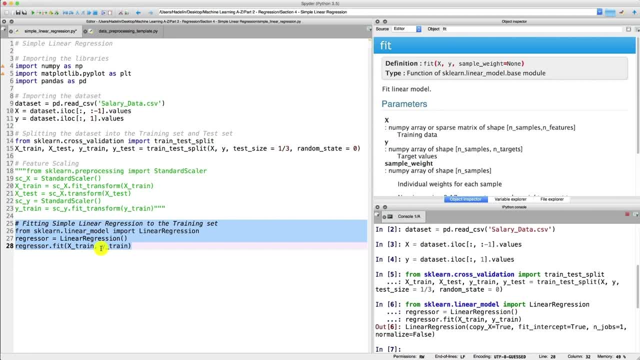 so that this machine, based on its learning experience, can then predict the salary with respect to the experience. so that's what machine learning is about. this is the most simple machine learning model and we just created it. and now that this simple linear regression, that is the machine itself. 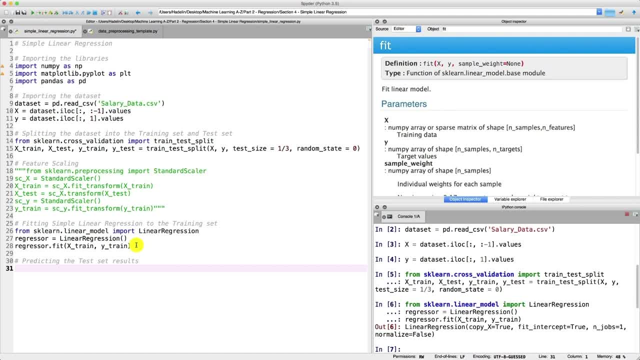 learned these correlations, we can see how it will predict some new observations, which will be the test set observations. and that's what we are going to do in this tutorial. we are going to see how our simple linear regression machine learned the correlations in a training set to see how it can predict. 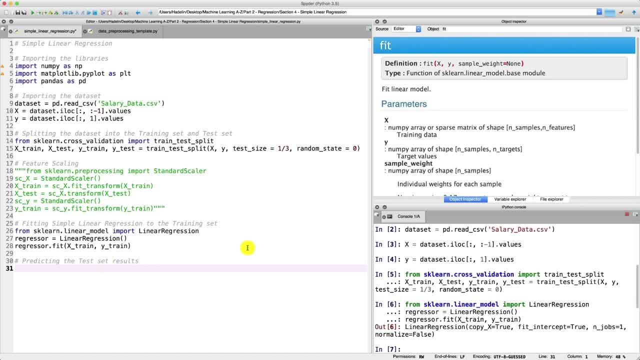 the test set observations which are new observations, because indeed our simple linear regression model didn't learn anything from the test set. so let's see how it can predict new observations and to do this, we will create a vector of predicted values. that is, we will create a vector. 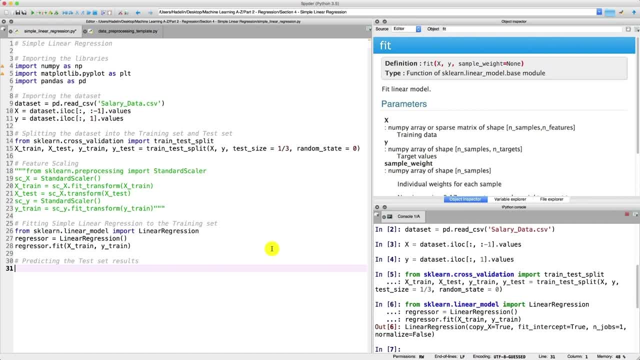 that will contain the predictions of the test set salary and we will put all these predicted salaries into a single vector that we will call ypred. so ypred- and this is going to be the same for all machine learning models that we will create- ypred is going to be the vector of predictions. 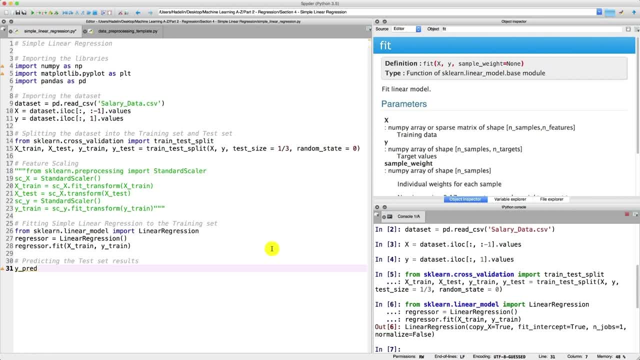 of the dependent variable and in this particular example, for simple linear regression. since the dependent variable is the salary, then that means that this vector will contain the predicted salaries for all the observations of our test set. so now let's create this vector of predictions. so here we will add equal. 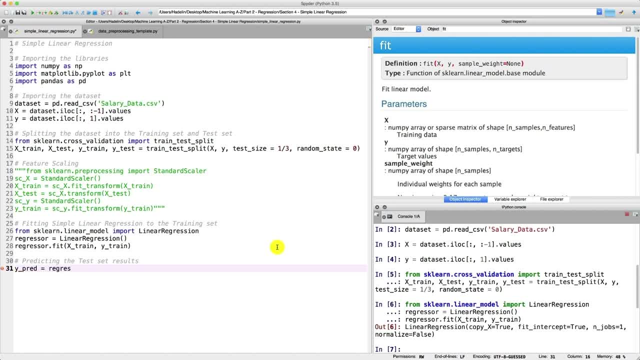 and now we will take our regressor that we created and trained on the training set, and again we are going to use a method of the linear regression class, but this time it's not going to be the fit method. it's going to be the predict method. 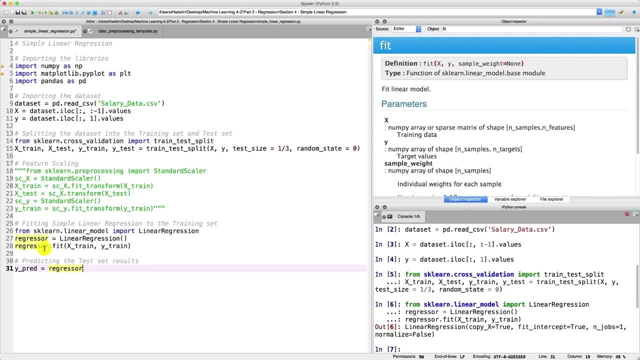 and the predict method, as you can guess, is a method that will make the predictions of the salary of some observations and therefore we will need to specify which observations we want to make the predictions. and so we will need to specify that we want to make the predictions of the test set. 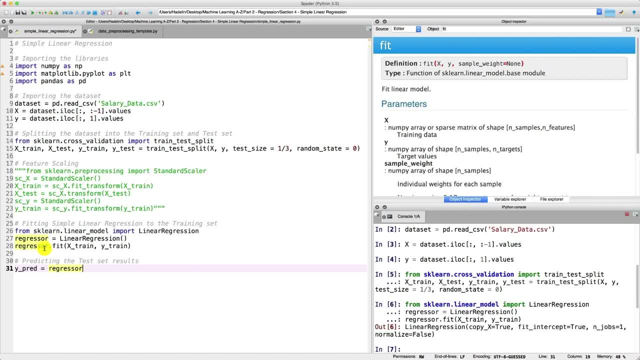 and so in this predict function we will input the test set. but you will see, so as always when we want to use a method, we add a little dot here and then we can choose the method here, as you can see. so before we use the fit method. 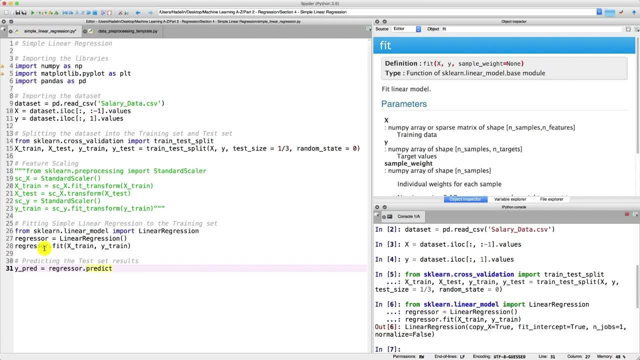 and this time we are using the predict method. so I just pressed enter and now we can input some parameter. so if we press command i to inspect the predict method, we get this and you can see that in the parameters. it says that we need to input only one parameter. 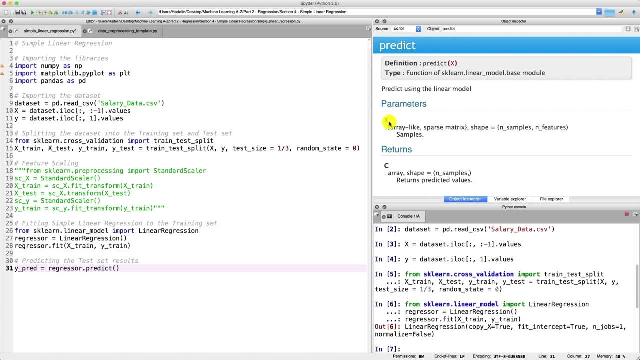 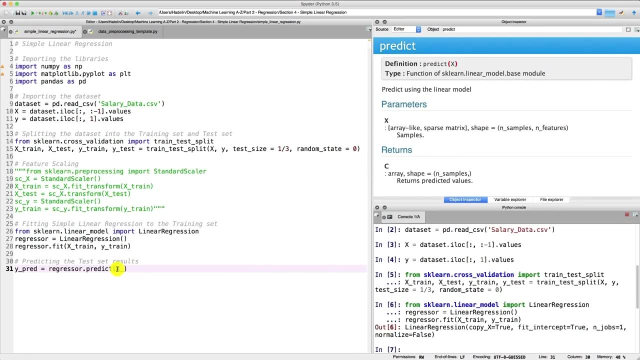 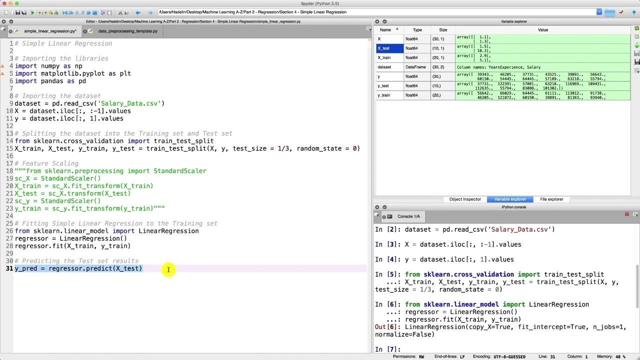 and that this parameter is x, and x is, of course, our matrix of features, of new observations, and therefore it's going to be xtest and let's select this line because now it's ready, the vector of predictions is ready to be built, execute and now we can see our ypred vector. 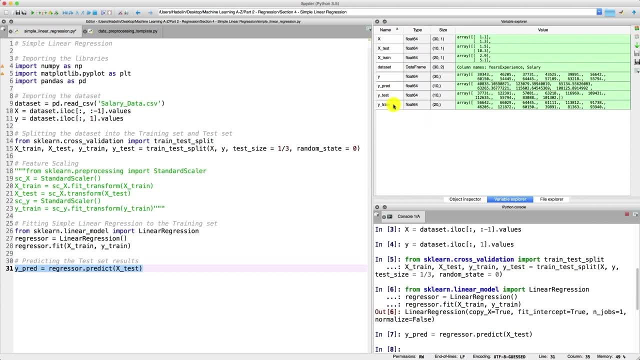 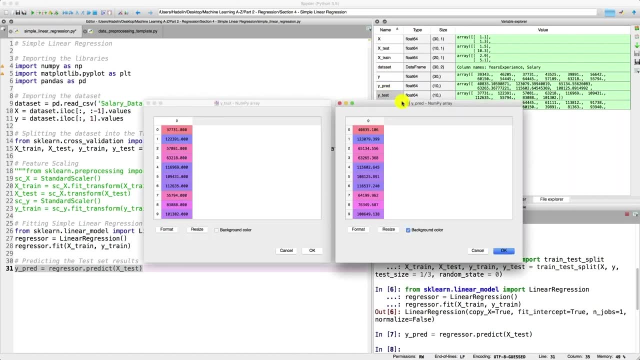 that actually appeared in the variables in the variable explorer. so let's have a look. here is ypred, and let's also open ytest to compare. alright, so now what's very important to understand is the distinction between ytest and ypred. so it's very simple. 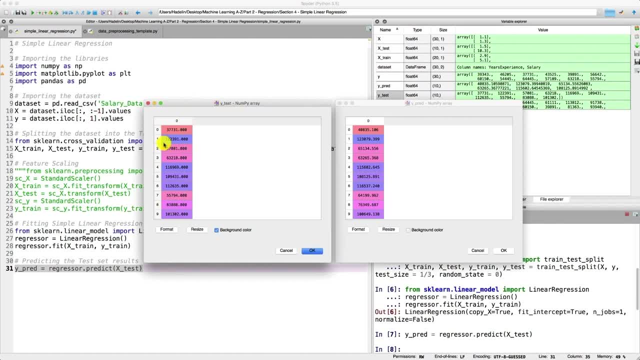 ytest is the real salaries of your 10 observations in a test set those 10 employees here really have in the company. and then those salaries here in the ypred vector are the predicted salaries. so that's the salaries of these 10 employees predicted by our simple linear regression model. 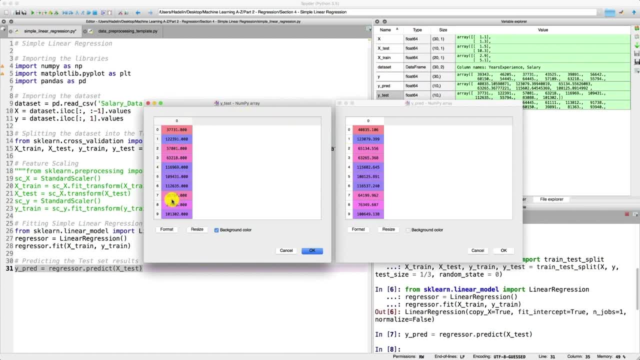 so, in short, ytest contains the real salaries and ypred contains the predicted salaries. so now what's interesting to do is to compare the real salaries to the predicted salaries. so, for example, let's take the first observation: so this real salary here and this predicted salary here. 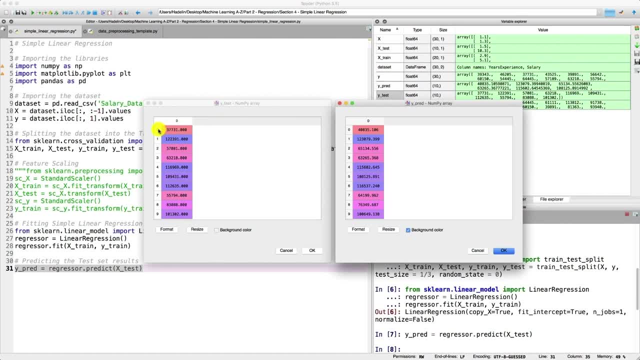 correspond to the same employee and we can see that this particular employee, indexed by zero, has a $37,000 salary- and that's his real salary- and our model predicted that this employee has a $40,000 salary, so the predicted salary is not too far. 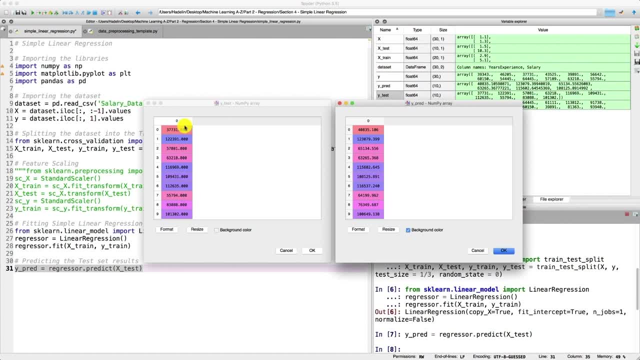 from the real salary and that actually makes a good prediction. we can have less good prediction, for example, if we look at the real salary of this employee here. well, it's real salary is $55,000 and our model predicted that this employee has a $64,000 salary. 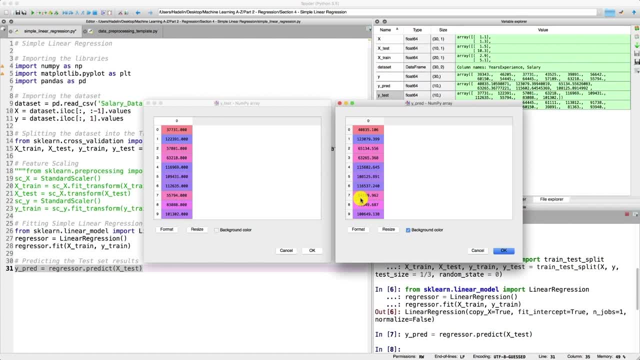 so it overestimated the salary, and you'll understand why it did that after when we look at the graphic results, you'll perfectly understand why, because you'll see that the simple linear regression is actually a straight line that is trying to be the closest as possible to the real observation point. 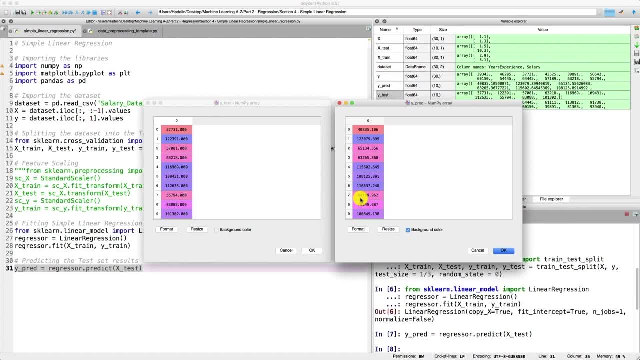 so you will see why it sometimes makes some predictions that are far from the reality. but then it can also make some great predictions, and that's the case for the last one, because the last employee of the test set has a $101,000 salary and our model predicted. 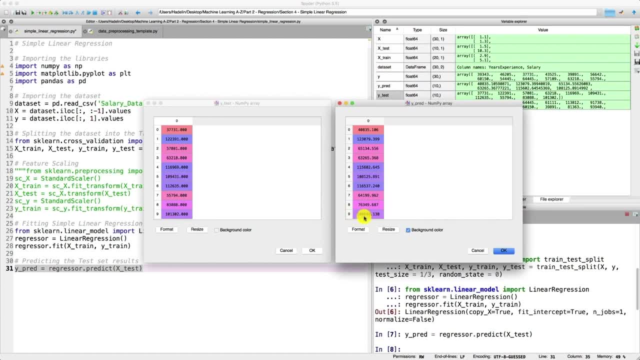 that this same employee has a $100,000- well, almost a $101,000- salary, so that's a very accurate prediction. ok, so let's click. ok, now that's the idea about the vector of predictions that we create here. all this will get a lot more clear. 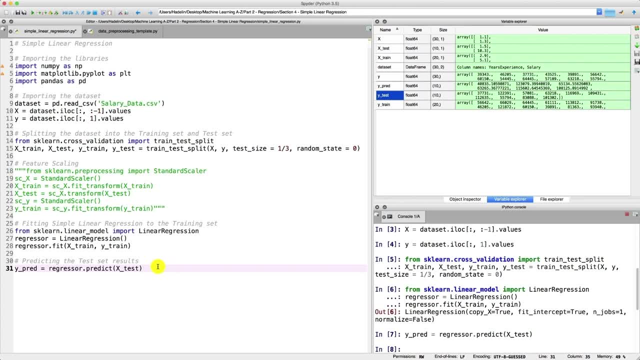 because we will visualize the result. we will visualize what's happening there between the truth and the predictions. we will build a plot where we'll have our true observation points. that means our employee with their real salaries, and then we will plot a straight, fitting line. that is going to be the simple linear regression line. 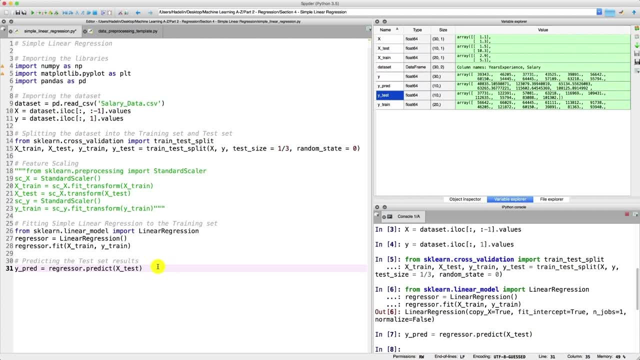 and on this line will actually be the predictions of our model for each of the employee. and now we are finally getting to the fun part, which is to visualize the training set and the test set result. so that means that we are going to plot, as well as the simple linear regression line, 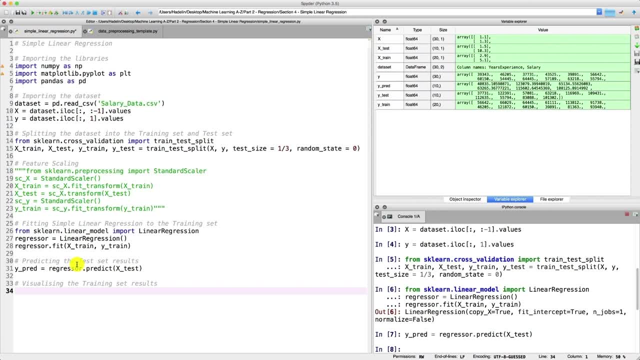 to see how there is this linear dependency and to see how the predictions of the simple linear model can be close to the real observations. so let's do this, let's plot these graphs and let's interpret the results. ok, so generally, to plot a graph in python. 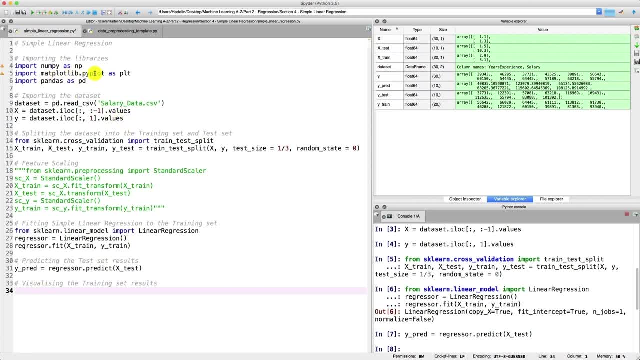 we are going to use this matplotlib pyplot library that we imported as an essential library in the preprocessing step. so it's already imported and we are ready to start plotting our graphs. so the first thing that we are going to do is to plot the real observation points. 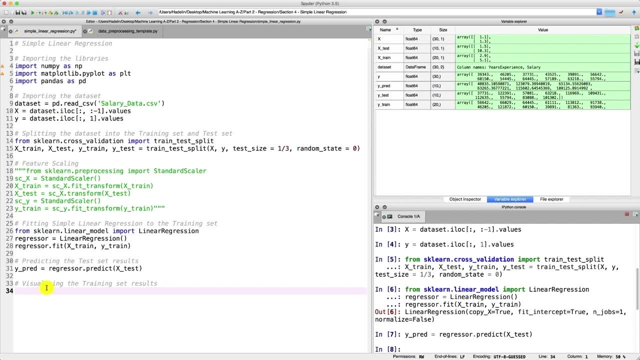 that is, the employees of the company, characterized by their number of years experience and their salary. that means that on the x-axis we will have the number of years of experience and on the y-axis we will have the salary. so let's do this. it's actually quite simple. 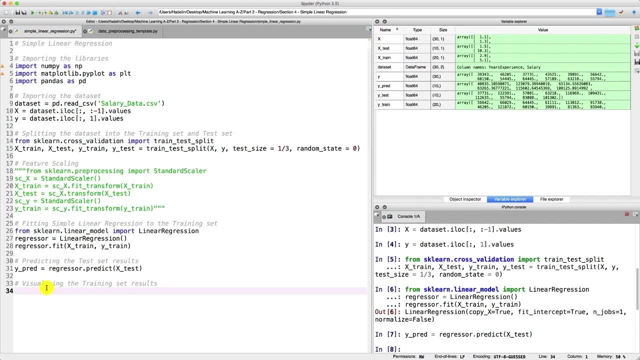 we need to use pltscatter, which is a function of pyplot. so you will see, it's actually quite simple. we just need to type pltscatter. then in parenthesis, we first need to input the x-coordinate of your observation points. so that's xtrain, because first we are starting with the training set. 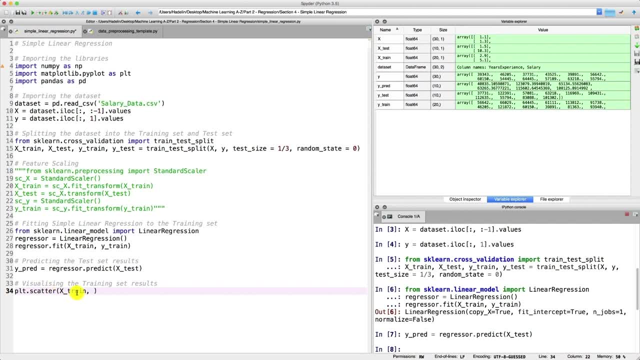 xtrain. so that's actually the x-coordinate of our observation points, because xtrain contains the number of years of experience. as you can see, these are the number of years of experience in xtrain. and now, what will be the y-coordinate? well, the y-coordinate will be: 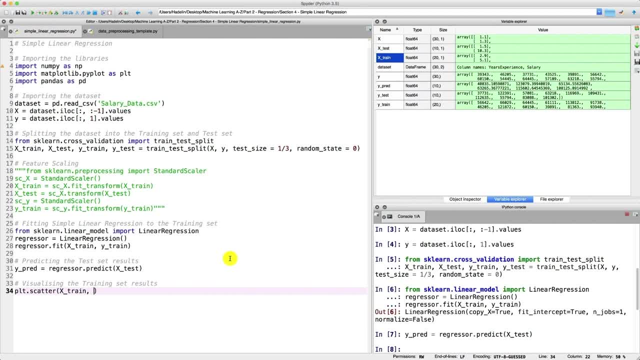 the real salaries that the employees have in the company and, of course, this is the salaries contained in the y-train vector. if we look at y-train here, these are the real salaries of our observation points, that is, of our employees in the company. so okay, that will be y-train. 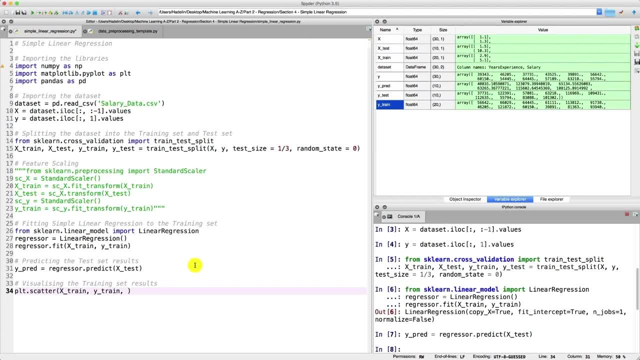 and then, since we will plot the observation points and also the regression line, it would be better to colorize in different colors those two entities, like the observation points in one color and the regression line in another color. so that's as you prefer. generally, what I like to choose is: 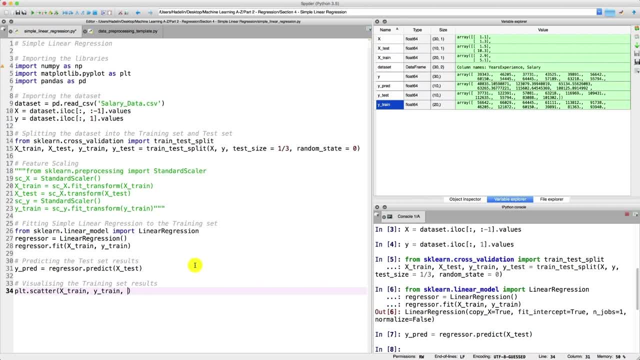 to colorize the observation points in red and the regression line in blue. so here I'll just choose: color equals red, alright, and that will plot all the observation points, the real values, and now what we are going to do is to plot the regression line, that is, the predictions. 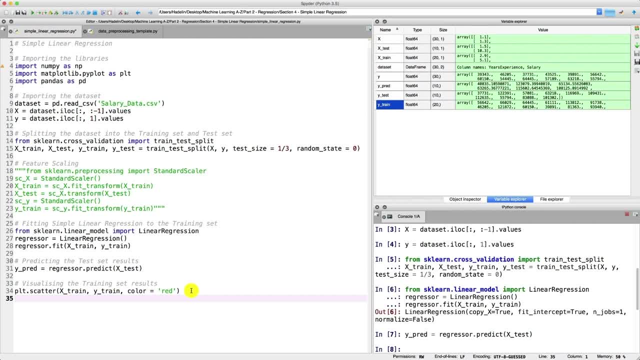 we are going to choose pltscatter, because we are not making a scatterplot of the points. we will use simply pltplot. and then, as usual, in pltplot we will first enter the x-coordinate of the points in the regression line and the y-coordinate, so the x-coordinate will be 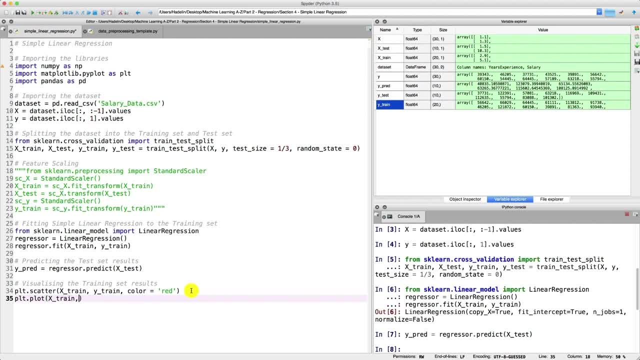 x-train as well, because you know, to plot a line we just need some x-coordinates of the line and then we will specify what the y-coordinates are. what do you think the y-coordinates of this regression line will be? well, it will be. 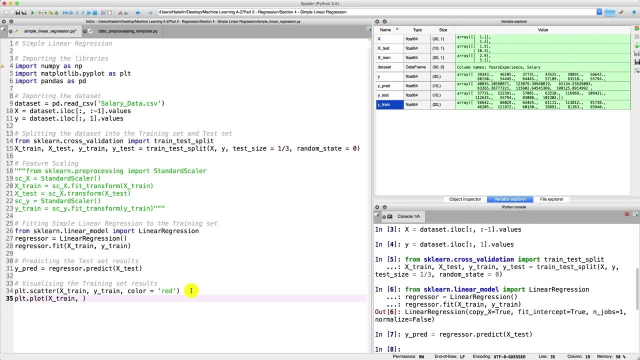 the predictions of the x-train numbers of years of experience. and the predictions of these numbers of years of experience in the training set in x-train are the predicted salaries of the x-train observations. so then, be careful, it's not y-pred, because y-pred are the predicted salaries. 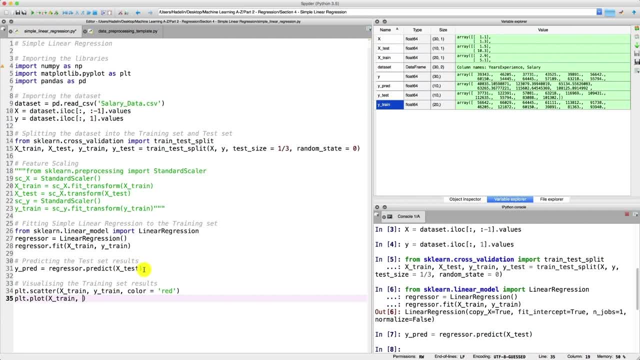 of the test set observations. here we have test set, but what we only need to do is to just copy this and paste it here, and here we will just need to replace x-test by x-train, because we want the predictions of the training set and not the test set. 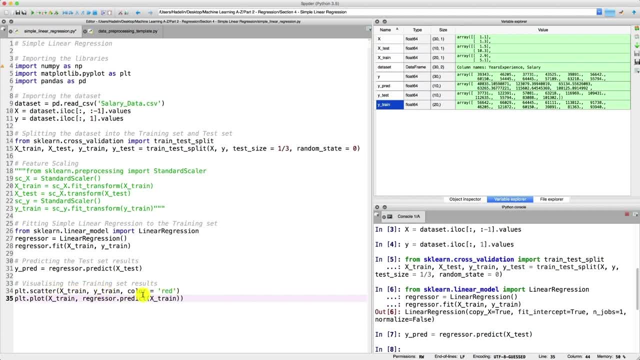 because here, you know, we want to compare the real salaries to the predicted salaries, but based on the same observations, that is, the observations of the training set. ok, so then we have our x-coordinates and our y-coordinates of the regression line, and now what do we need? 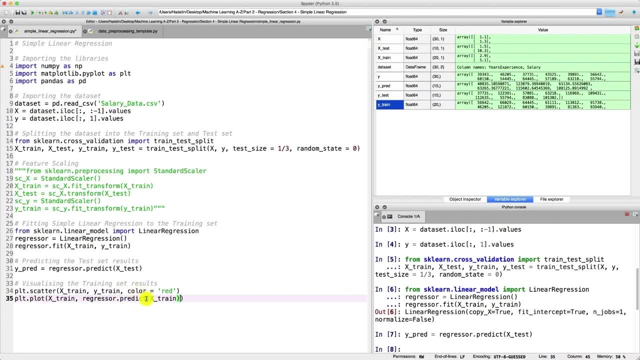 a color? yes, because we want to make the distinction between the observation points above and our regression line. so since we chose red for the observation points here, we'll choose blue, or you can choose whatever you want. that's just my personal preference, but you're welcome to try something different. 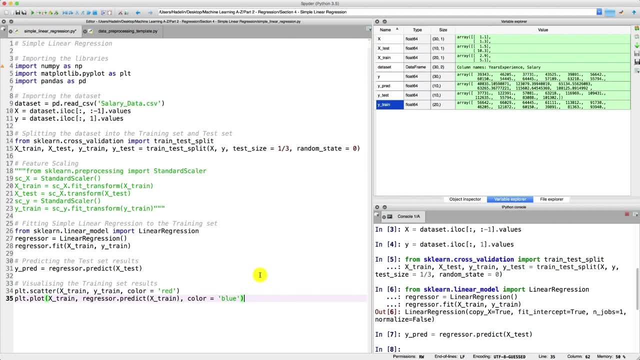 and here it is. this Zeichen line plots the simple linear regression fitting line to our training set. ok, now we'll just improve our plot by giving a title, a label at the x-axis, a label to the y-axis. ready, so let's do this, let's add a title. 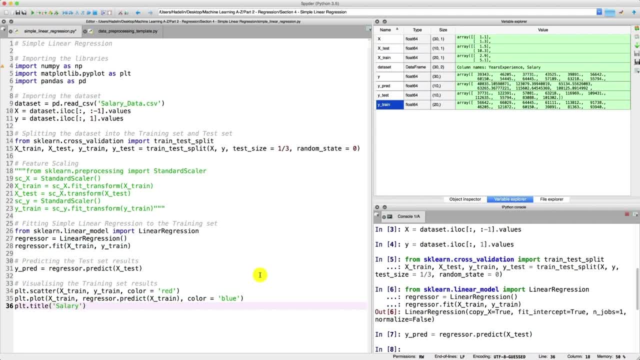 it's plttitle. let's give salary vs experience, because we want to see the relationship between the salary and the experience. and here let's just add training set in parenthesis to specify that we're plotting the training set results, because then we'll do the same for the test set results. 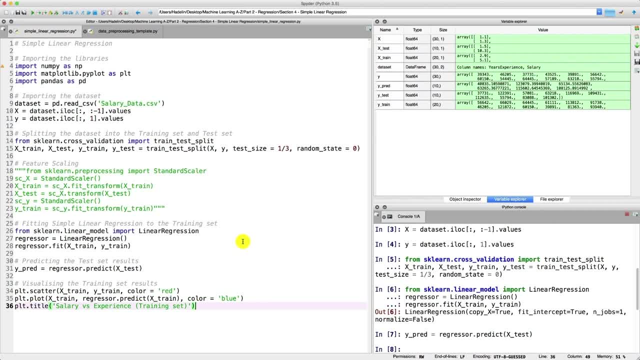 just to make the distinction. and that's it for the title. great, now let's add a label to the x-axis. so to do this we just need to add the command pltxlabel, and then let's call our x-axis years of experience, because on the x-axis are the numbers of years of experience. 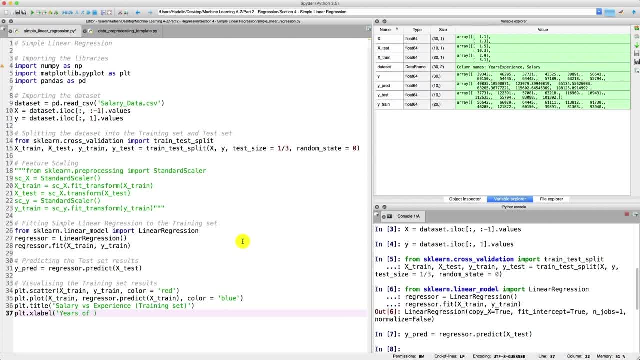 so years of experience here. it is great. and now let's add the y-axis. so this time it's going to be pltylabel and then parenthesis: salary- alright, great. and then we just need to add a final line. it's pltshow with parenthesis, and that's to specify that. 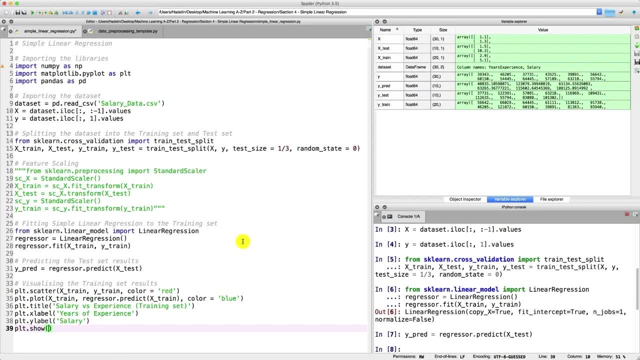 it's the end of the graph and that we're ready to plot it. ok, so now it should be good. we have our observation points, we have our regression line. thanks to pltplot, we have a title labels to our axis, so it should be all fine. 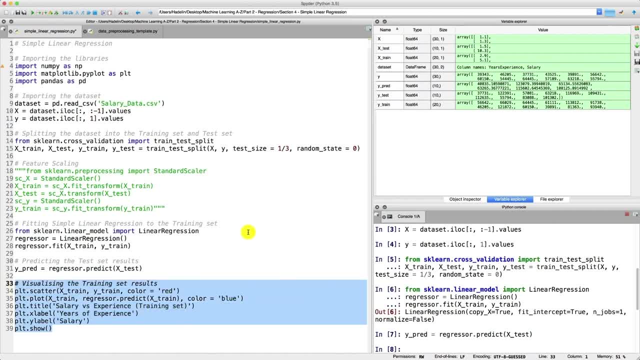 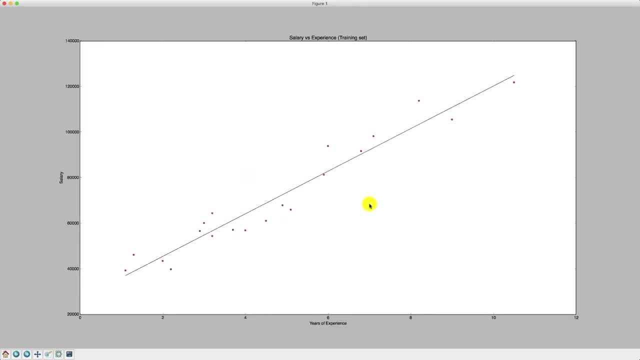 let's try to select this and execute. press command and control plus enter to execute, and here is our graph. great, let's enlarge this alright. so ok, the first really important distinction to understand is that we need to make the distinction between the real values and the predicted values. 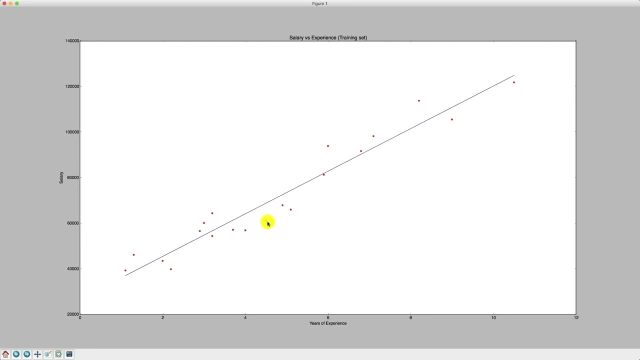 so the real values are red observation points, all these red points here. these contain the real values of our employees, that is ok, their years of experience, but then their real salary, the salary they really have in the company. and then the predicted values are on this blue, simple linear regression line. 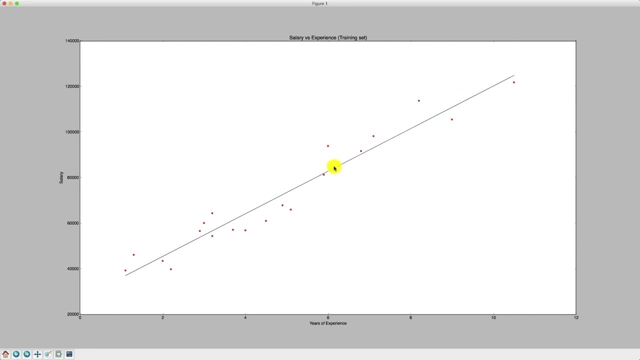 and by predicted values I mean the predicted salaries, which are the projections of the points of this line to the y-axis. so, for example, if we take this observation point here, that corresponds to an employee that has 4 years of experience and a salary about $55,000. 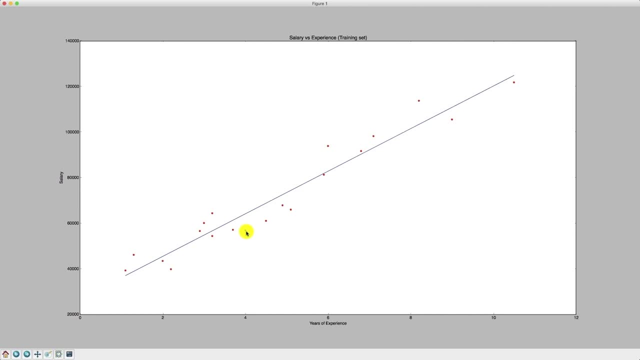 so that's its real salary. but then to get the predicted salary of this employee, we need to first project this point on the regression line and then project again to the y-axis to get the predicted salary, which is then $60,000. so for this observation point, 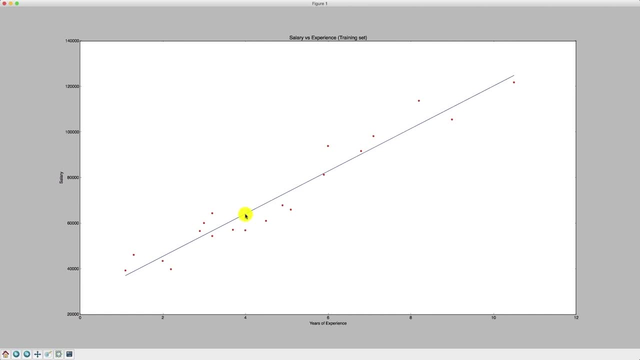 the real value for its salary is $55,000 and the predicted value for its salary is $60,000. so that's the first really important distinction to make. now, what's interesting to see is that there is clearly a linear dependency between the salary and the years of experience because, as we can see, 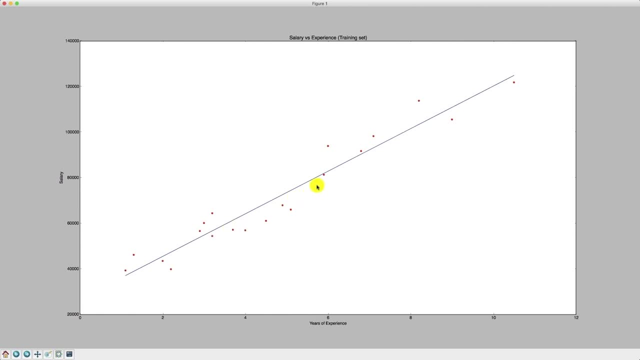 our regression line is approaching quite well all our observation points. you know, if we had some points everywhere, then our regression model could fit a straight line, but it would be far from our observation points. but here, since it's approaching quite well the points, then that means that there is linear dependency. 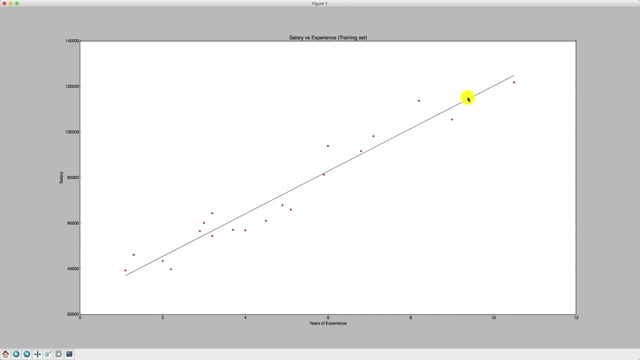 and that's why we could fit a good, simple linear regression model that gives good predictions. and speaking of predictions, we have some accurate predictions, for example, this one: we can see that the real salary is close to the predicted salary. this one, too, this one, is a very accurate prediction. 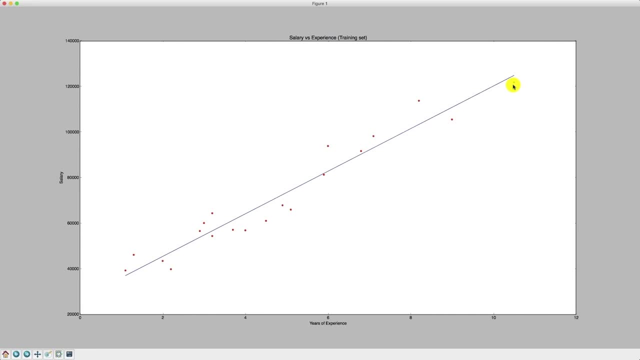 the prediction is almost perfect, and this one as well, and then, of course, we have some less accurate predictions, because this is not a 100% linear dependency. so of course, for example, this real salary here is further from the predicted salary which is here. so here, as you can see, that's the predicted salary. 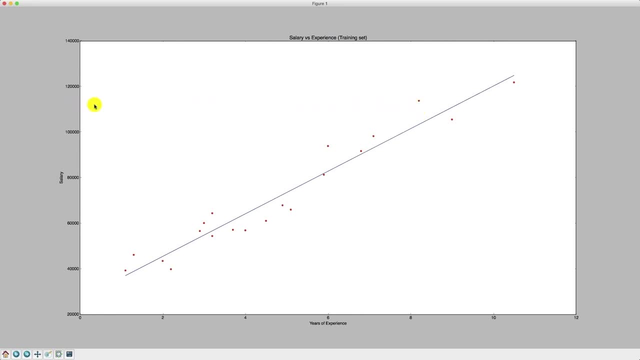 for this particular employee, and that's the real salary, and same for this employee, and this one as well, this one as well. and now the third thing that is actually important and that we have to keep in mind each time we make a model, is that these are the observations of the training set. 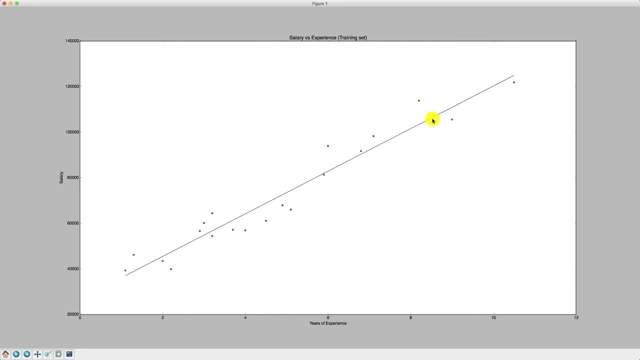 so these are the results of our simple linear regression model, but which was trained on all these red points here, on all these red observation points. here let's see how this simple linear regression blue line can approach new observations, and these new observations will actually be the test set observations. 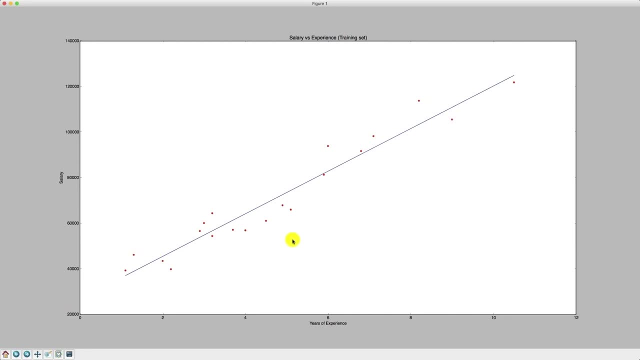 these are new observations because our model didn't learn on these test set observations. so what we will do next is we will plot the same kind of graph. we will keep this blue regression line because this is the regression line that was trained on the training set, so we don't want to change that. 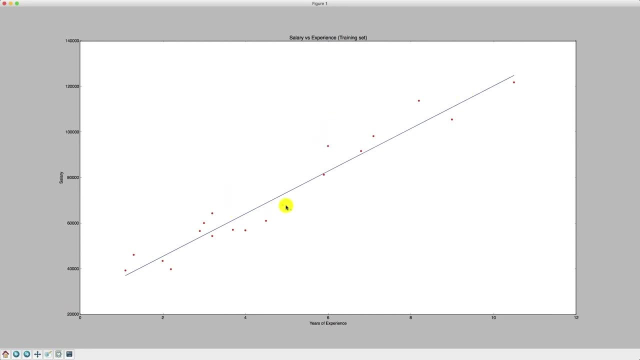 however, we will plot some new red points here. these are the training set observation points, and we will plot in the second graph the test set observation points. so let's do this and let's see how our simple linear regression line can predict some new observations. so what we will do is we will 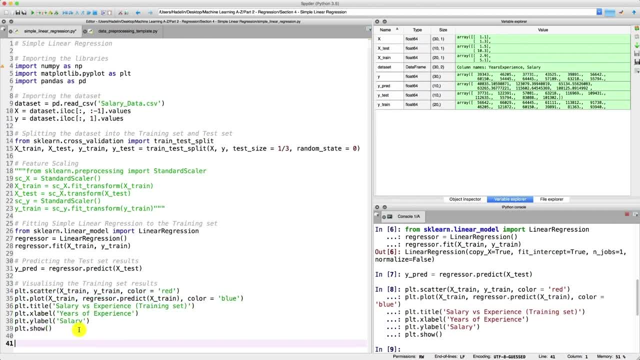 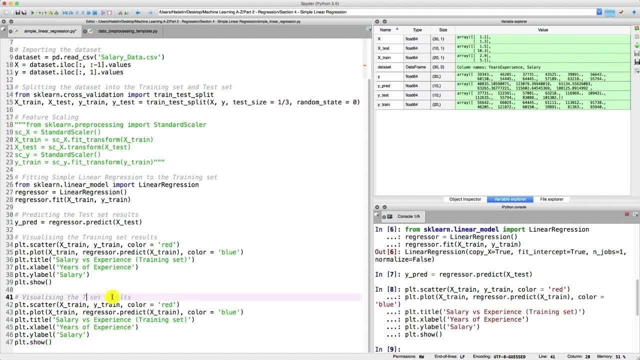 copy this actually and paste it here, because you will see that we will only have a few things to change. ok, so first let's change the section title here and specify that we are now visualizing the test set results. ok, and here let's specify also in the title of the plot: 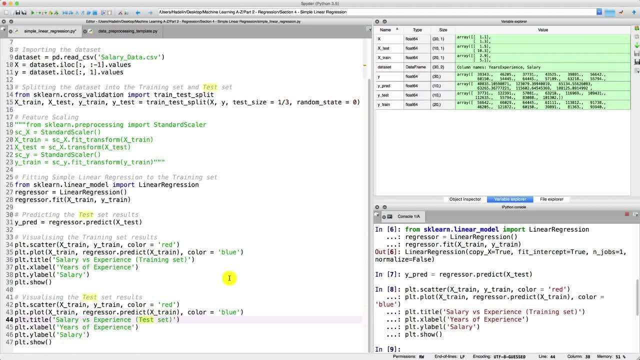 that we are now plotting the test set results. great, and now, what do we need to choose? ok, so in the first line, the first line is pltscatter. that plots our observation points. and now, since we are interested in looking at the observation points of the test set, 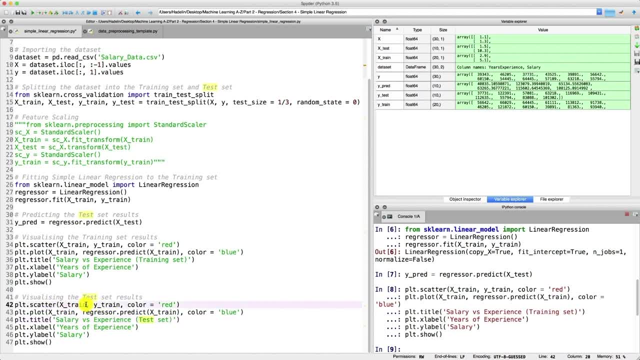 here it won't be xtrain and ytrain, it will be xtest and ytest, because xtest and ytest are the coordinates of the observation points of the test set. and then something very important to understand here: do you think that in the second line, pltplot- 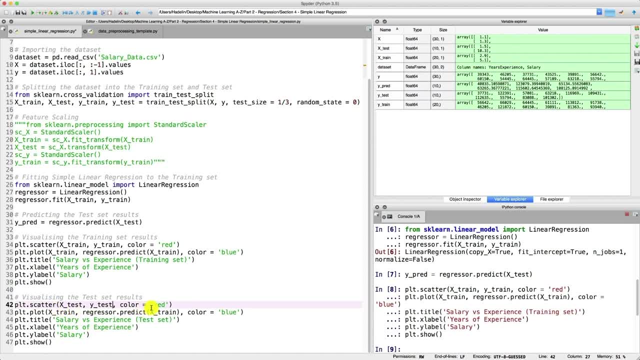 do you think we need to change xtrain here and here by xtest? and the answer is no, because our regressor is already trained on the training set. so whether we keep here the training set or replace by test set, we will obtain the same simple linear. 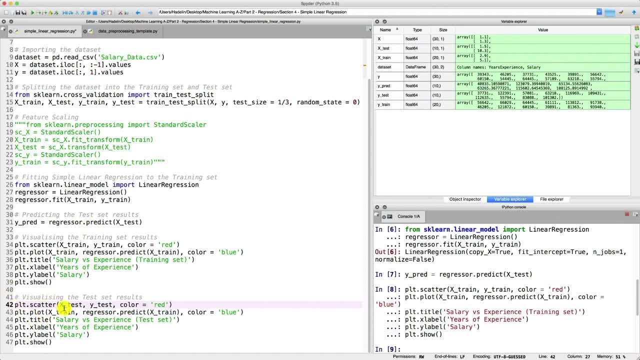 regression line. indeed, if we replaced here xtrain by xtest, we would just build some new points of the same regression line corresponding to the new predictions of the test set, observation points, because when we trained our simple linear regressor on the training set, we obtained one. 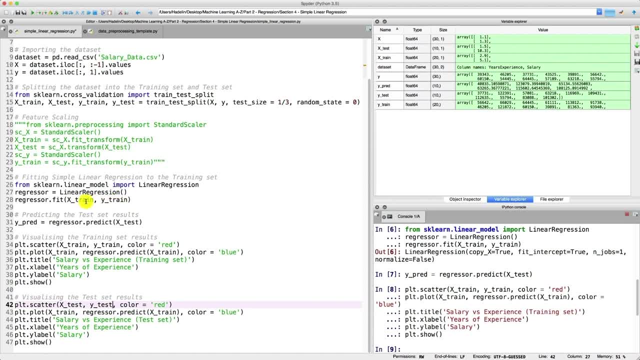 unique model equation, which is the simple linear equation itself, and therefore, whether we build the regression line here by predicting the training set points or the test set points, well, since this predictions result from the same unique, simple linear equation, we will get the same regression line. so actually this is: 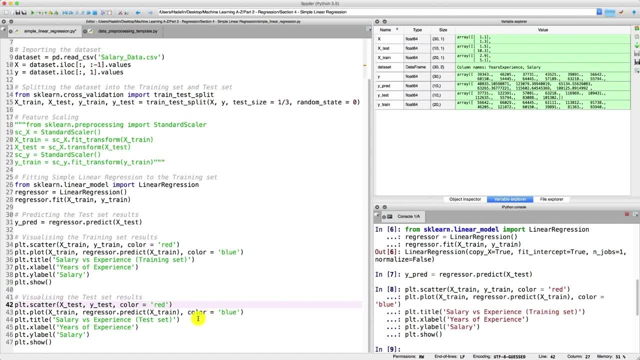 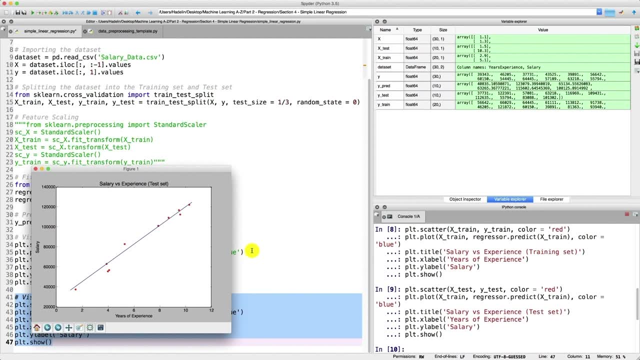 already now we are ready to plot the test set result, so let's do this. i'll select this and press command and control plus enter to execute. and here are the test set results. so let's enlarge this, okay. so these are the test set results, so be careful. 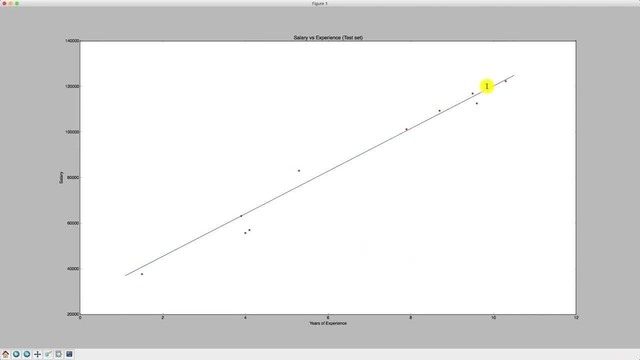 this blue regression line is the blue regression line that we had in our previous plot in the training set results. so that's the same line, because that's our simple linear regression model, trained on the training set. but then these red points, here are new points, these are the observation points of the test set. 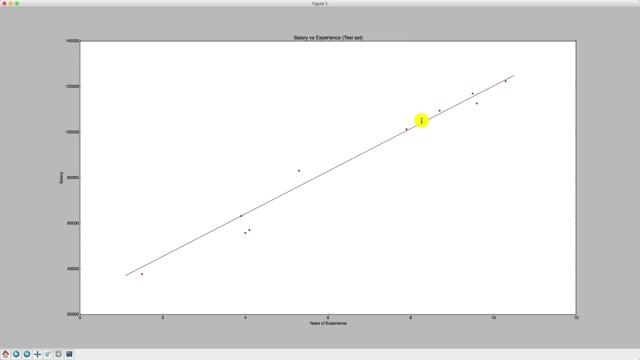 whereas before it was the observation points of the training set. so it's important to understand all this, and now let's interpret and let's give the final verdict. well, this is actually really good, because these are new observations and our simple linear regression model is making some very good job.